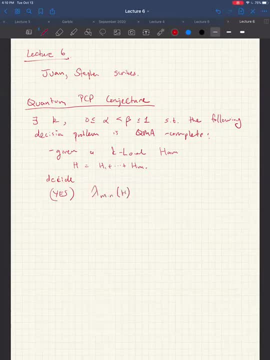 the ground energy of this local Hamiltonian is at most this constant alpha times the number of terms. Okay, and in the no instance you have that the ground energy is above beta times m. So so this is the conjecture, and just recall that what we do know is true is this quantum Cook Levin theorem. 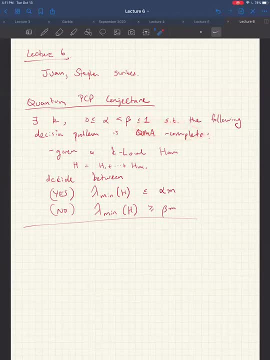 which you know. the problem that is QMA complete is the same problem, except that the difference between the yes and no instances is just some invert, some inverse polynomial amount, so something that's like a vanishingly small number. but the quantum PCP conjecture is stating that in fact it's still QMA hard when the difference 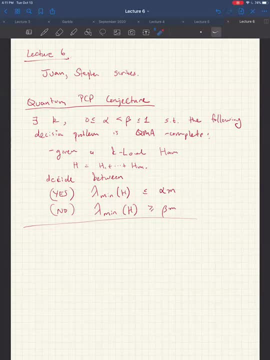 between the yes and no instances are is very large, something that's growing as a, as a function of the, the number of terms or the number of particles involved in the system. so we don't know. this is true and you know I sort of went into this informal discussion of 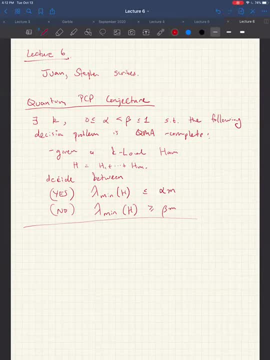 what would the implications be if this PCP conjecture were true? namely, it would have implications possibly for many body physics. all right, and we had some pretty good discussion about that last time, and, and we're going to move on to the next slide and we'll continue it a little longer for today, 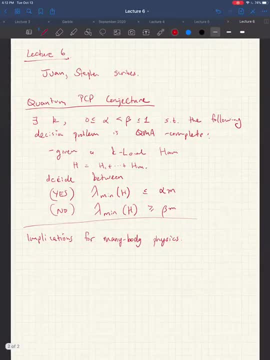 so intuitively. if this quantum PCP conjecture were true and we also made some very natural complexity theory assumptions, so let's see: quantum PCP plus some complexity assumptions, it would imply things like the existence of local Hamiltonians who's- I'll use some scare quotes here- room temperature. 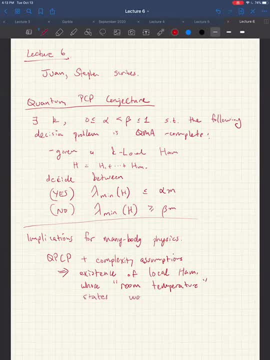 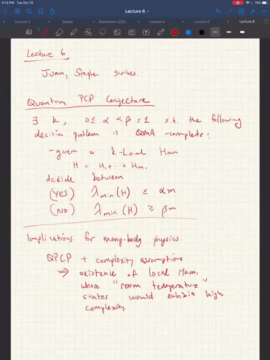 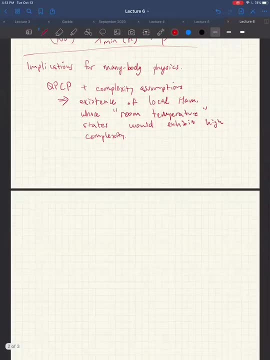 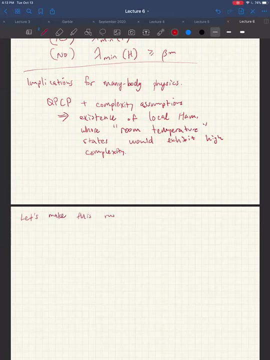 so what I want to do right now is actually just make this the statement and and this formulation a little more precise, so so we know what we're talking about. so the first thing I want to do is I want to define what I mean, uh, by high complexity. so I have to introduce some sort of measure of 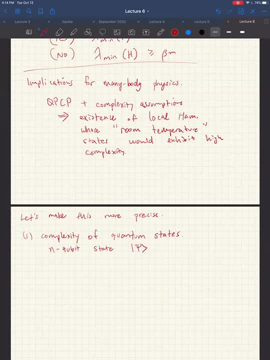 complexity of quantum states, then I'm going to define its complexity to be the minimum depth of a circuit that's required to create this state. This is the where, if you took the circuit and you applied it to say, some initial state like the all zero state, you would actually get the desired target state. 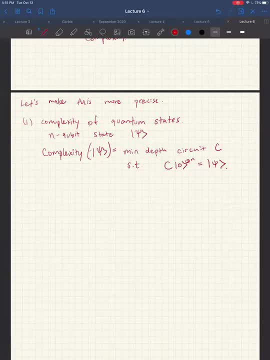 So let's get a feel, for you know this measure, Henry, is this in the basis where psi is the easiest to prepare, Because I can prepare the plus state as complexity one and like applying Hadamard on every qubit. but if I just move to the x basis, then I 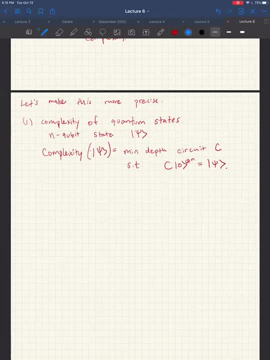 don't need to do anything and I'm already in the plus state. So here I guess we're just assuming for simplicity that we're starting in the all zero state. so to create the plus state, like you mentioned, you would have to apply a layer of Hadamards, so the depth would be one. So I guess, 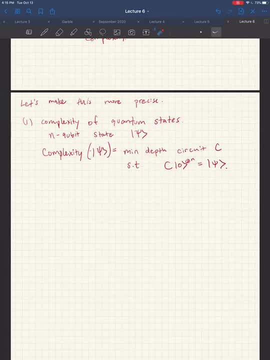 it's just sort of you know. it's in the same way that for a quantum circuit you have to fix some particular gate set and you just stick with it. For this definition, you pick some initial starting state and in this case we'll pick the all zero state. You could also define it to be the all plus state, for example. 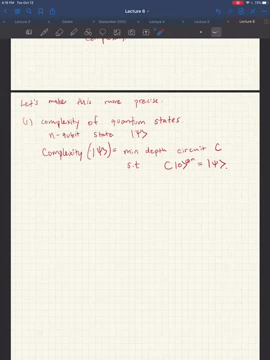 and it wouldn't really fundamentally change how you use this measure. But I mean more than the complexity of a quantum state. the complexity depends on the on the basis you chose to describe your problem in. So, for example, you could map your problem to a quantum computer working in the diagonal basis of the Hamiltonian. 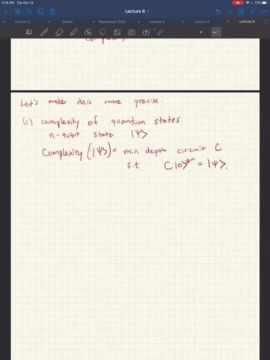 already, then all the eigenstates would just be basis states, basically. But if you work in some other basis, then these eigenstates are highly entangled. So when you say that the complexity of space is the only thing that you can do, then you can't do that. 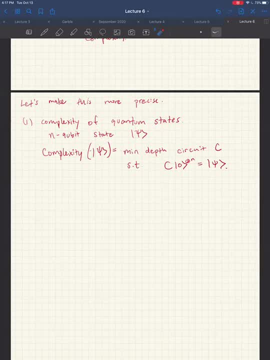 So is it in the basis where it's the easiest to compare? or I mean, does it change anything I see? Well, I guess you know whenever you're talking about a quantum state, you're going to fix some, like when you're talking about n-qubit states, right, so you have some particular. 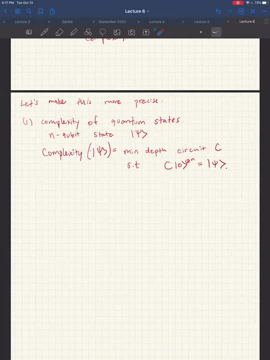 representation for the basis of each qubit. and then if you have a state psi, then on n-qubits, then of course there's always a basis in which your state psi looks like the all zero state. but that's, I mean somehow that doesn't you know. that would be too easy, right? so I guess the point is maybe just the complexity. 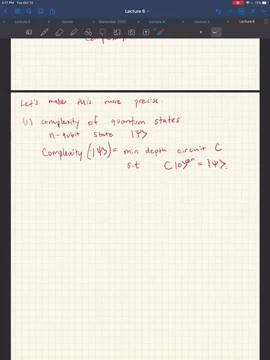 depends on the basis you look at. Yeah, it definitely depends on the basis. I guess the point is, you know you fix a basis for each of the qubits and then you just leave that fixed and then all your states you talk about are with respect to that basis. Okay, great thanks. 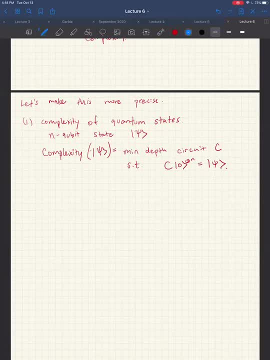 I guess one can also phrase this definition in algebraic terms, like the minimal amount of unitary operations you need to apply on the one zero, zero, zero, zero, zero, zero to get the vector that represents your state. or am I not getting this right? Yes, that's exactly right. So here's circuit. yeah, actually I should. I should have said in: 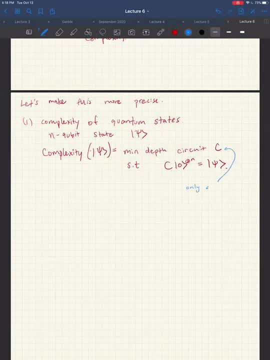 this circuit we only allow, say, two qubit gates. oh right, otherwise, if your circuit could be an arbitrary unitary, then in some sense every state can be prepared in depth, Because you would just have a unitary that maps to that state. so maybe this is related to what. 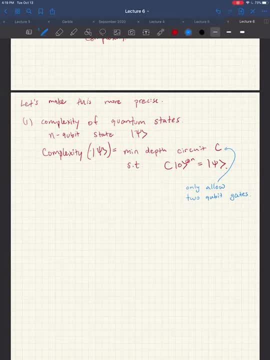 Alexandre was asking, but here we're only allowing two qubit gates. let's, let's say it's an arbitrary two qubit gate, that you can pick any one, but they have to be two qubits. and the question is given those, you know, what's the minimum number of layers? do you need to prepare the target state psi? 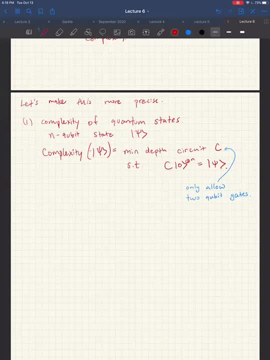 Okay so. so let's just look at a couple examples to get a feel for for this measure. So any product state, so let's say your state psi, is just a tensor product of individual qubits. right, so each of these psi i's are going to be just one qubit states. 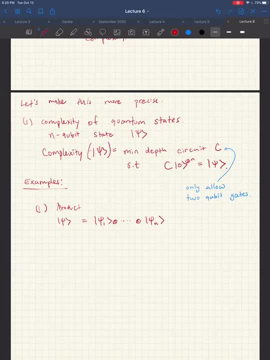 then? then what's the circuit, complexity of this, of such a state, Right, at least you know, asymptotically this: this will be okay, the max of the complexity of each of them, Good, and, and the complexity of each state will be, you know, it'll be as Abhinav says, order one, it's a constant. 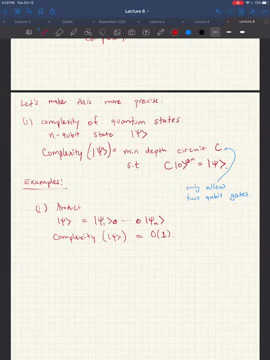 right, because basically you just have a gate, prepare each state, but you do it all in parallel, right? so so you have the the all zeros and we also allow one qubit gates too. Okay, we just have each of these unitaries will be one qubit state. 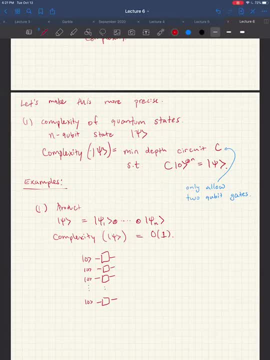 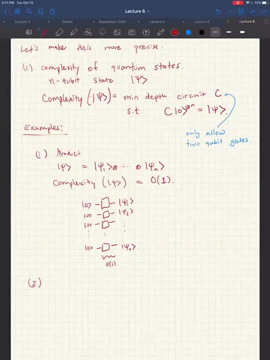 So these unitaries will be the one that maps, you know, the state zero to the state psi. one psi i. So you only need one layer. so this is order one. Okay, so product states have a trivial circuit complexity. so whenever it has order one, we just say this is trivial. 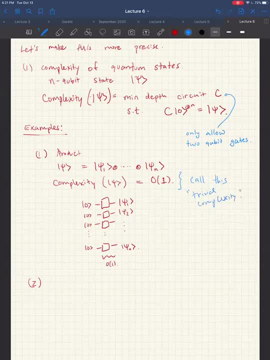 Okay. so so we're kind of saying that product states or unentangled states are not that interesting. What's a more interesting state? Well, let's look at what's called the cat state, also known as the ghz state. So this is just the equal superposition between all zeros and all ones. 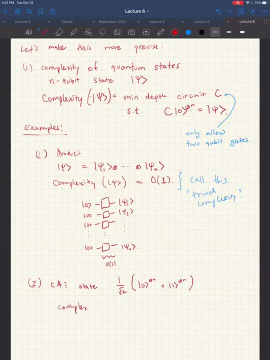 Does anyone have an idea about what's the complexity of of this state? What's? what depth circuit do you need to to create this? Okay, Abhinav says n plus one. that is an upper bound, but you can do better. I have an intuition that says log n, but I'm really not not not sure. it's like I don't know. 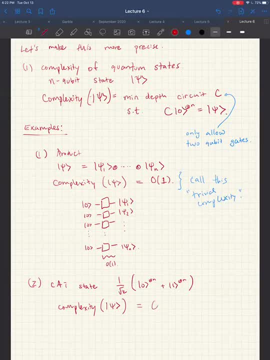 So. so log n is indeed the right answer. You can build the state in log n depth. That's very good, Basically, you, you just kind of, actually, you know, maybe I'll leave it as an exercise for you to to work out on your own. 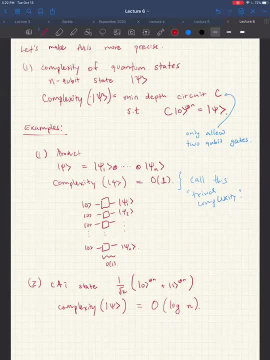 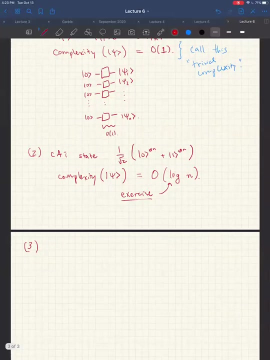 Actually, this is something that you'll see on your problem set. so okay, okay. so so this is slightly more interesting. this cat state has some entanglement right And this circuit complexity kind of captures it And, you know, the final example that we'll see is is something that's on the 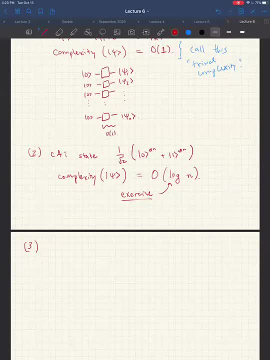 way, other extreme of the spectrum, which is if you take a random quantum state, so that you know there's a well-defined notion in which you can sample an n-qubit quantum state uniformly at random, And this thing is is going to be a super complicated mess. 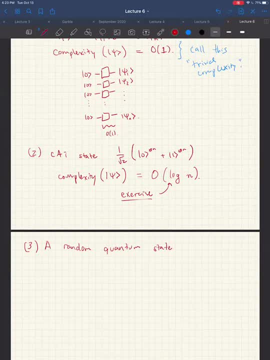 It's going to have maximal circuit complexity with very high probability. So a random quantum state with high probability satisfies its complexity, being it's actually going to be exponentially large in n Right And- and this is the, the maximum amount Right you can approximately prepare or actually, as you know, you can build an. 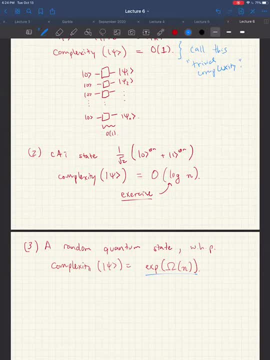 arbitrarily good approximation of any quantum state you want with exponential size circuits. What's the omega for? The omega is to just hide some constants. that Yeah, I mean. um, you know, there's some constant in front of the n. It's not going to be like e to the n exactly, but there's gonna be some constant there. 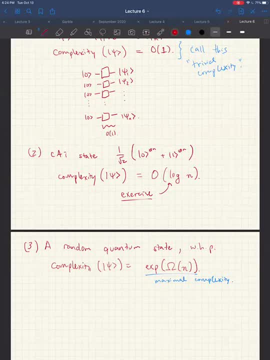 I mean, once we're here, what's the difference between like, omega and big O notation? Oh uh, good question. So, um, basically, big O means like at most, and then omega means at least up to some constant. So, um, right, so, like you know, f is equal to O of g. if f is less than uh, c times g, roughly speaking. 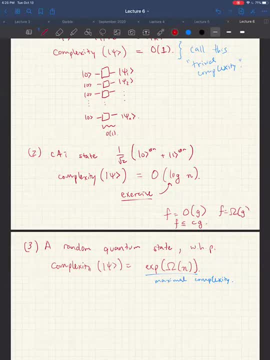 Whereas if uh f is omega of g, then then this basically means there is some constant- we don't we're not necessarily keeping track- but there is some universal constant- for which f is greater than c times g. So f and g are functions here that that you know go off into. 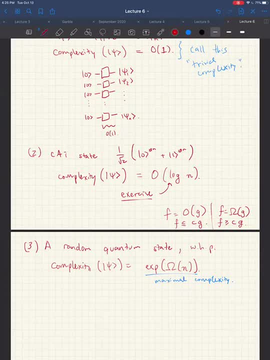 infinity. Henry, I have a quick question. Yeah, I'm I'm kind of surprised by this exponential uh thing, because I- my memory of this might be mistaken, but I thought that you can create an arbitrary unitary on n qubits in order: n squared qubits. 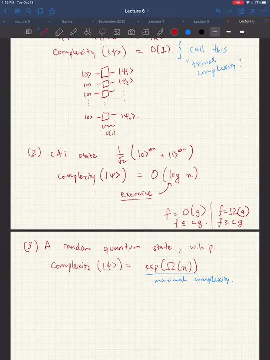 Just the combination of all single qubit rotations And all, uh, two qubit controlled rotations. Hmm, so here, um, we're talking about the, the, so you're talking about the number of qubits required, um, but uh, oh, we're talking about circuit. um, yeah, circuit, uh size. so so definitely circuits, uh. 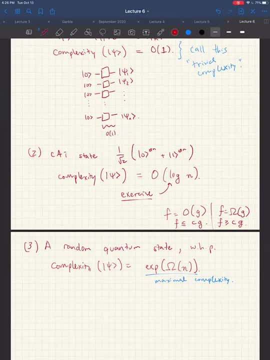 like I mean, if you just sort of like roughly count the number of unitaries, uh, I mean there's an infinite number of them, but like, if you sort of discretize, then the number of unitaries, uh is is going to be um doubly exponential in n. 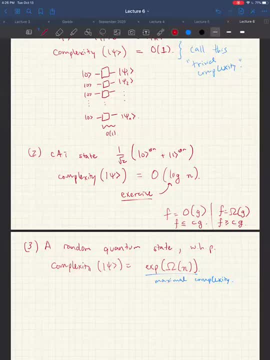 So so basically that that means, like in general the, the number of gates you would need to to produce a generic unitary would be exponential in n. Does this bound assume a, a gate set like Clifford, plus t gate set, or, if you're going to do it in a? 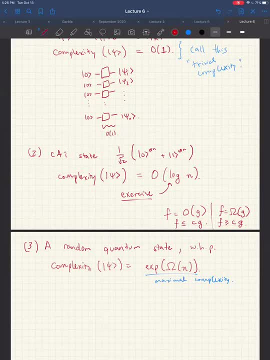 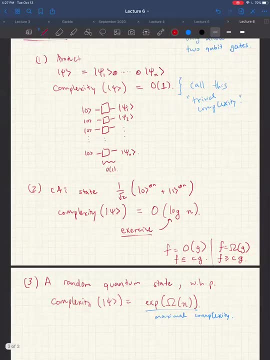 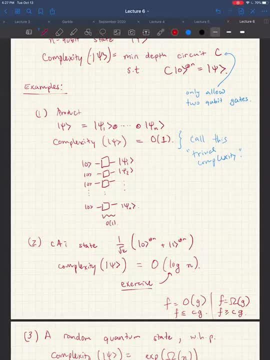 cubic gates, so it can be continuous. Um, uh. if you restrict to Clifford and t it, it'd be the same thing it? the difference is just: uh, you can only implement unitaries approximately rather than exactly, whereas if you allow arbitrary two qubit gates and you can actually, with sufficiently many gates, implement. 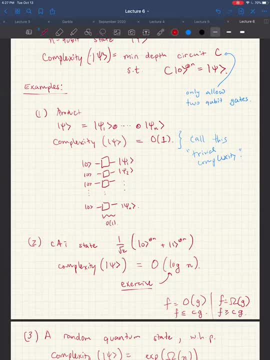 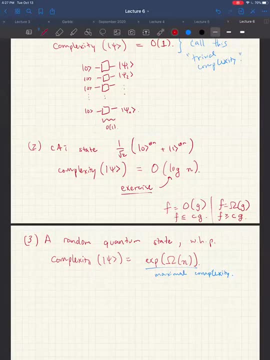 every unitary exactly, But qualitatively, that these bounds will all be the same. Okay, so, Henry, can you say something more about how you sample a random quantum state? Mm-hmm, How do you sample one? Well, I guess the 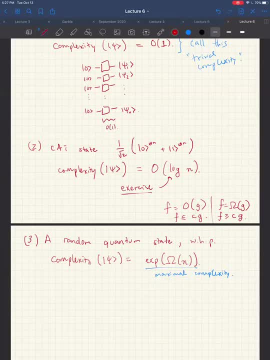 the technical definition is that there's, you know, the set of all quantum states on n qubits is. you can think of it as like the unit sphere in dimensions 2 to the n, And so this is a. you know, it's a compact set and you can define something. 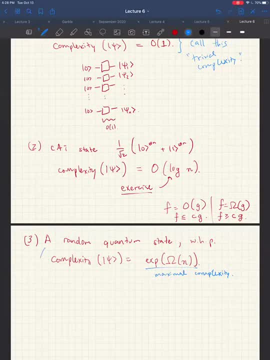 called the Haar measure. I forget what's the. you know what's the notation. I know it's like projective space on c2 to the n or you know something like that. You know there's a, there's like a. 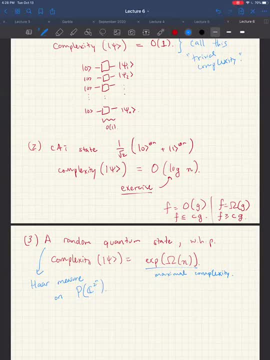 rotationally invariant measure on this which you can sample from. If you're saying, like, what is a mathematical procedure to actually sample from it, One way is to. one way to do it is you can just pick a vector of length 2 to the n. 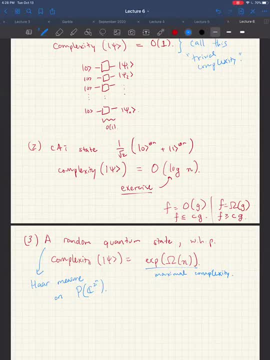 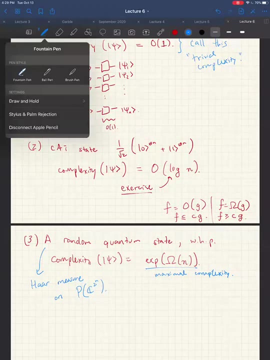 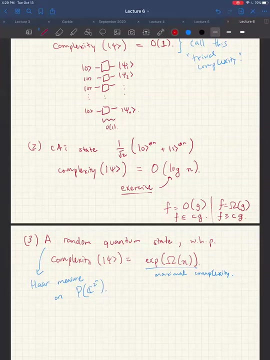 and each entry, you independently pick a random Gaussian and then you just divide it into the form of this vector and then you'll get a uniformly random unit vector. I see, Thanks. Okay, So so this complexity measure, it's like, has high dynamic range, right Like it. 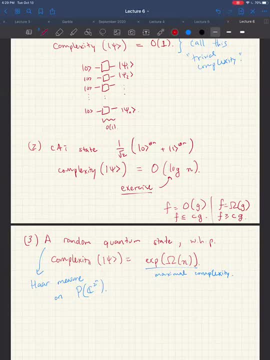 you know it can be everywhere, anywhere from, like you know, zero all the way to exponential and n, And so there's this huge range. right for possibilities, Right. And so what you can do is you can have a very complex complexity measure and then this one has like a high 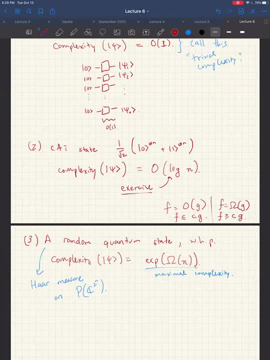 dynamic range, right, Like it, you know, it can be everywhere, anywhere from, like you know, zero all the way to exponential and n, And so there's this huge range right for possibilities for the complexity of a quantum state, and we can think of the complexity. 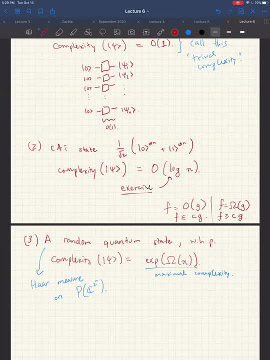 of a measure as capturing how complicated is the entanglement inherent in the state. The complexity is measured by. you know you get to give someone hands you the state and you get to try to pick what is the shortest possible circuit I can try to build in order. 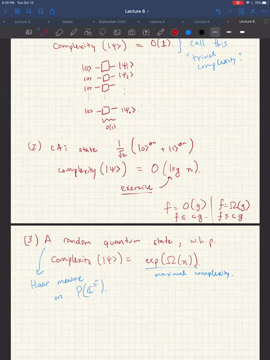 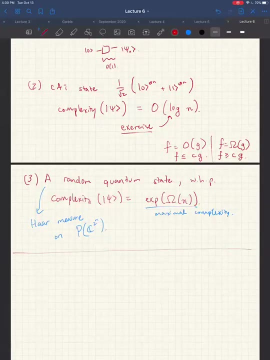 to get this state, And if the shortest circuit still requires exponential depth or super-polynomial depth, then it tells you that you know it's really, you know complicated And you know we can think that the states that at least we can get our hands on in this. 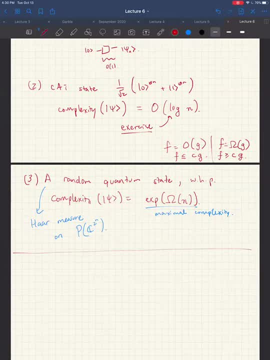 universe efficiently will be the ones that have polynomial complexity. So you know. so, morally speaking, the physically relevant States, you know, the ones that you could hope to observe in a lab or something, are going to be the ones that have polynomial complexity. 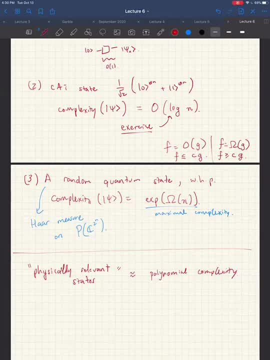 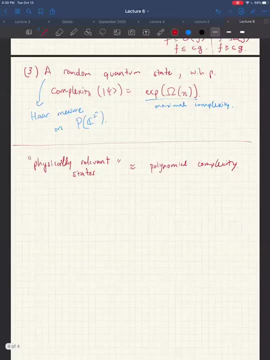 Because if it has more than polynomial complexity, you have no hope in general of ever seeing it in front of you. Why is that, Henry? So, yeah, I mean also, you know, I'm, I'm, You know, the last couple lectures I'm making a lot of these moral statements but feel 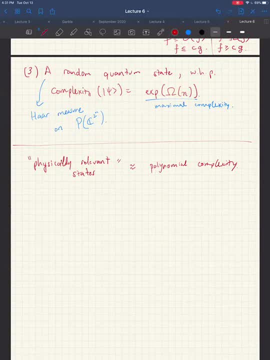 free to fight back. So basically, you know we're equating polynomial time as what's efficiently doable in a reasonable amount of time. And you know, asymptotically we can think of, you know, things that take exponential time. 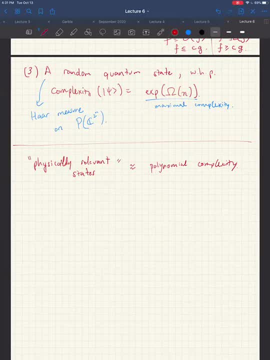 So let's say you have a 300 qubit state, Something that's exponential, And 300 is 2 to the 300, you know that that's. there haven't been that many nanoseconds or or plank times in the history of the universe, right? 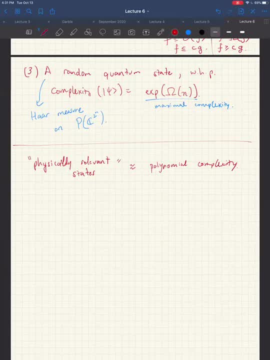 So if something requires a circuit of depth 2 to the 300 in order to prepare, we can be pretty sure that there is no physical process in this universe that could have produced it right. So so you know, we don't expect to see such states. 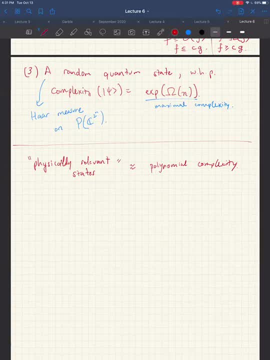 Around. Well, there is no deterministic process that produces it. Maybe there is randomness in the world, Like I don't know. Yeah, In the natural world do you have that everything goes like evolves by two qubit unitaries, Or can you possibly have that? 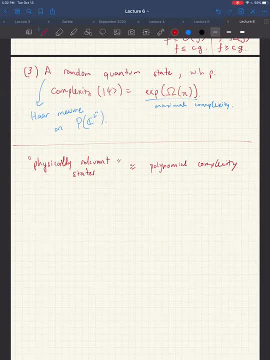 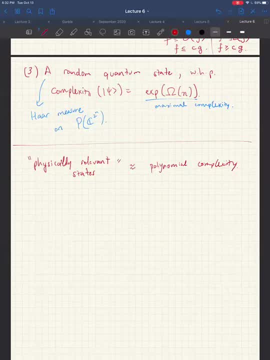 Yeah, Yeah, Yeah Yeah. These are great questions, so Let's see, let me answer. you've also sorry, you've always question: was what was your question here? Like I don't know if this question may make sense, but like what? maybe random in some. 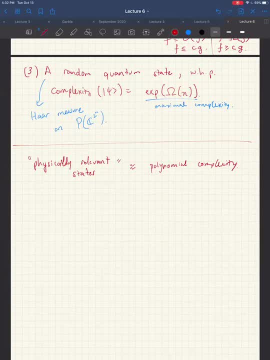 sense and that's if Right. So maybe there's some random, maybe there's some random process out, You know, in some galaxies, somewhere that you know just spits out these states with exponential complexity, that's possible. But then you know, if you try to imagine. 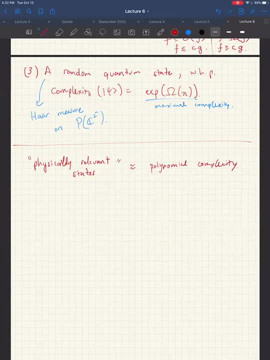 well, what is this random process? It's, it's some. I mean, ultimately, we think if you assume that you know the, that the laws of nature obey quantum mechanics and obey, maybe, the standard model of physics, then whatever random process, it's just really occurring because of local. 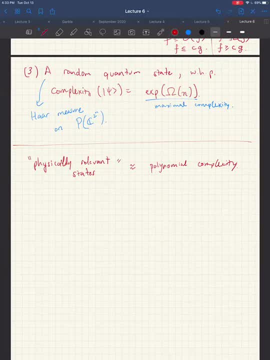 forces that are interacting in some ways and some particles are bumping into each other and and you know the, you know things are being measured and so on. But all of this, we believe, can be simulated by a quantum computer. right This, this is just a belief. 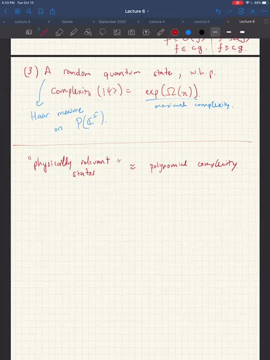 right, This is called the quantum church Turing thesis, that any physical process that exists in the universe you can simulate efficiently using a quantum computer. So, um you know, whatever crazy thing is going on in the next galaxy over? uh, we're. 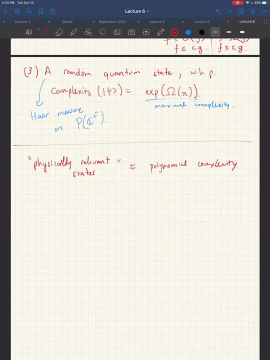 we're going to assume that that um, it could have been simulated by uh polynomials on quantum computers. So so, therefore, all the states that this galaxy could have produced um should have polynomial complexity Right, And and maybe that uh, and that also answers. 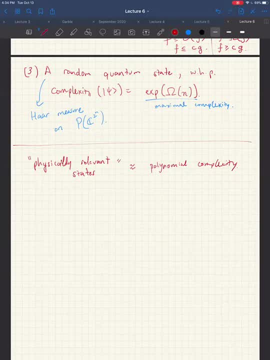 maybe answers Hugh's question. Uh LO, you were asking about the two qubit gates, right? So so we think that, um, yeah, And and when I say quantum computer, I mean one that that operates using two qubit gates. 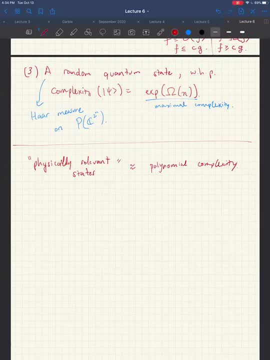 I feel like this could blow up with recursion, though Like one. the wave function of the universe, say, includes perhaps in some portion of it the wave function of a quantum computer that is solving a problem that is QMA complete. Uh, right, That's a physically possible process. Uh, and so this would seem to imply that it's. 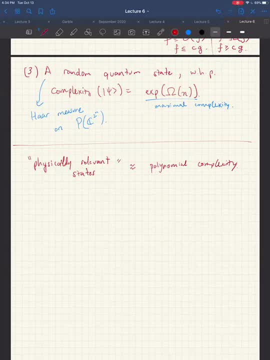 polynomially hard to simulate the solving of a QMA complete problem, which looks to me like QMA equals BQP, Right? So um, so we have to be careful what we mean by. what does it mean for something to solve Right, So we have to be careful what we mean by. what does it mean for? 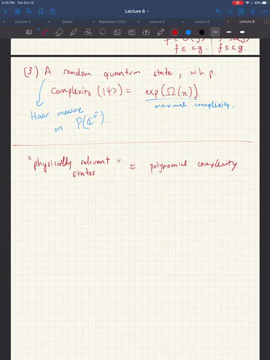 to solve a QMA complete problem. And here- this is where it's important to remember- are we solving a specific instance, Because we can always get lucky. For example, like, if you want to solve an NP complete problem or a QMA complete problem, you can just run, you know. 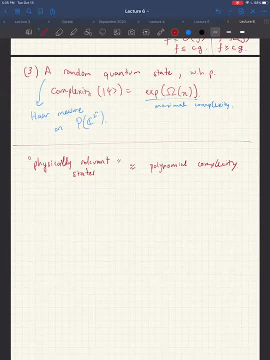 your favorite algorithm to try to solve it And you know, maybe you'll make the correct guesses and you'll find the correct solution. But in general we don't expect such an algorithm to succeed on all possible instances. So let me say it again: Solving a QMA complete problem. 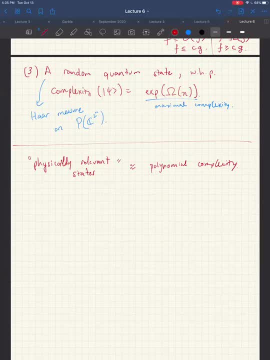 it means that you can solve it in polynomial time, no matter what instance you give to it, And that's not something that you can necessarily. So, okay, well, I don't know if the answer to your question. So if you're saying, like you know, 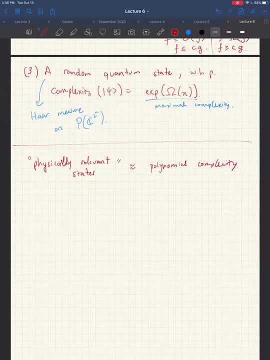 this wave function of: if you're simulating the universe and inside this universe there's a computer, you can solve it. So if you're saying like, you know this wave function of. if you're saying like, you know this wave function of if you're saying like, you know this wave function. 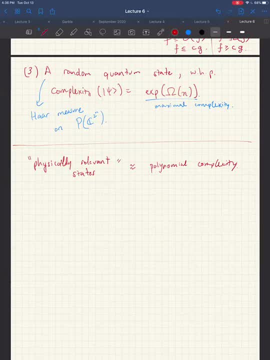 that happens to solve an instance of a QMA complete problem. there's no contradiction there, because it doesn't mean that we've found a polynomial time algorithm to solve all instances of, say, the local Hamiltonian problem. Oh yeah, right, Because a compute 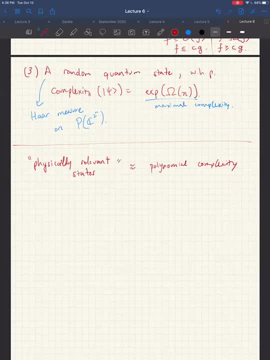 like any instance could have some tailor-made algorithm solving it, And that drops the complexity down considerably Right? So you know, in that sense, when we talk about solving problems we really mean that can you solve all instances or like a large, you know an infinite number of possible instances And that's. 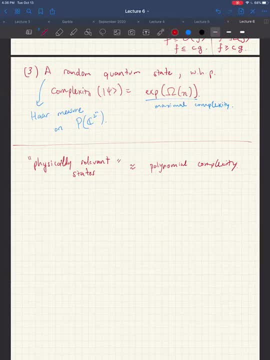 when it makes sense to say whether you're solving it in polynomial time or not. Actually, you know I should. you know maybe this is familiar to a lot of people, but you know when I use the terms polynomial or exponential, this only makes sense when you're talking about a growth in the 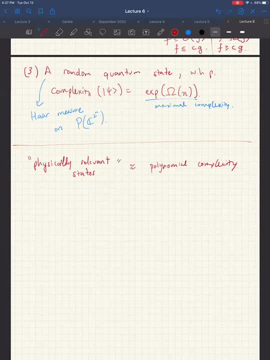 number of you know there's some asymptotic quantity Like, for example. it doesn't make sense to say: is the number 100 polynomial or exponential, right? That's like meaningless. It's only what you're saying as a function of something that you imagine is going off to infinity, like the number. 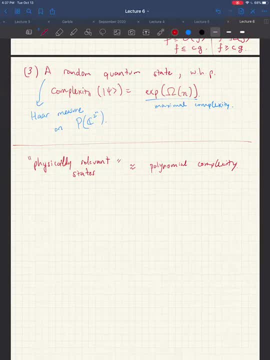 of particles or something like that. One more pushback on this: physically relevant states equals polynomial complexity piece Related to what someone was asking before about this kind of being basis dependent. So I agree that for our analysis of like a particular of a quantum computer or quantum algorithm or something we fix, you know the gates that are. 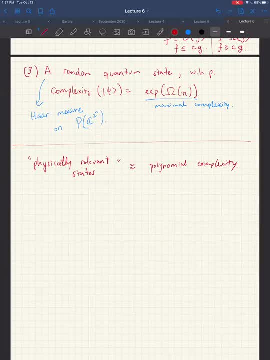 allowed, we fix the basis we're working in. But it might be kind of like the universe is working in, working in some other basis and produces some state in polynomial time in that basis. But that's kind of one that in our basis would require an exponentially large circuit to create. 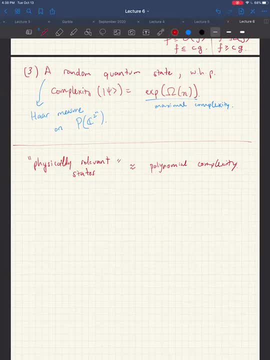 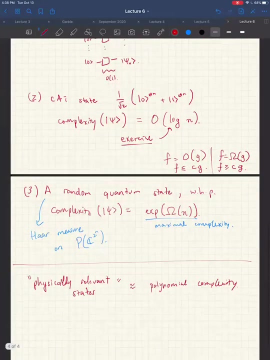 Okay, yeah, that's a good point you raise. So here it's true that if you're allowed arbitrary changes of basis, then you can. something that would have been easy in one basis could be difficult in another, and vice versa. But actually we sort of think that we only should allow. 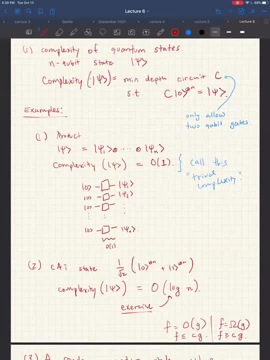 basis changes that are local. like you can, you should really only be able to change the basis of, you know, individual cubes. Okay, You can change the basis of 300 qubits separately, but you shouldn't be able to like completely. 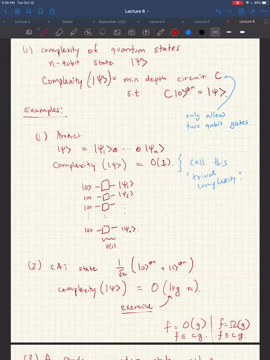 change the basis in which you're like, you know the entire basis of your laboratory, Or you know, change the entire basis of 300 qubits all at the same time. So I hear the point you're trying to make, But that's kind of like that's our choice When we 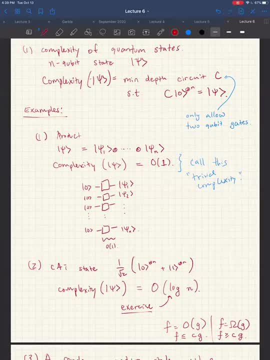 decide to analyze a quantum system. it's our choice of how to factor the larger Hilbert space into a smaller one. Right, That's right. So I guess then you know the question I have for you is: is there a physically, is there like some experiment that you can run where you know you have? 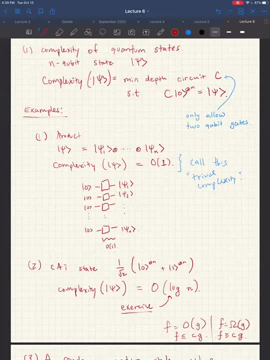 a bunch of different particles that you sort of factored out as like: okay, there's a particle here, here, here, here, here, but then I can do a large change of basis that simultaneously, right, Makes sort of smears out. all these different you know qubits together into something that's. 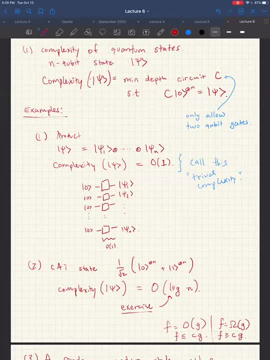 completely different And as far as I can tell it's, I don't think we know of physical processes that that look like that. Fair enough, Although I don't know of any reason why there couldn't be. Yeah, so if there is, then okay. 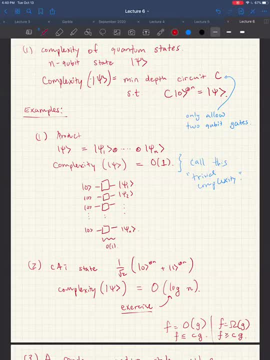 so the point is, if there is something like that, then you might hope to possibly take advantage of that to to gain some sort of speed up. But I think what the- you know this, this church Turing thesis that I mentioned- sort of posits or assumes that such a thing. 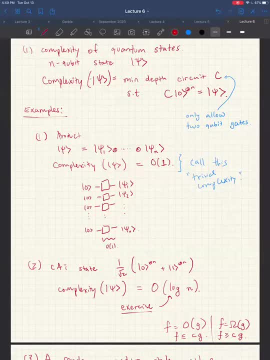 is, it's not really possible. But you know, if you, you can always prove it wrong by saying: hey look, I found a physical process that does allow me to to make this change of basis. So sorry, just back to what you were saying before. So you were saying that we believe. 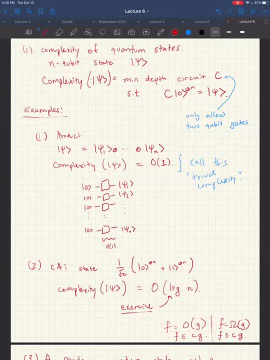 that any like physical quantum system that evolve, that like like any, if it runs quote unquote quickly then we can simulate it in like quote unquote polynomial time with like two qubit gates. like efficient physical quantum processes can be like efficiently simulated. 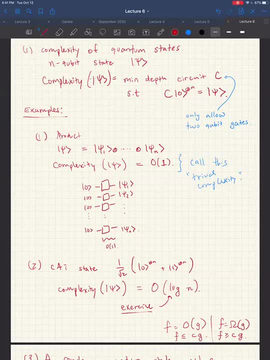 by these two qubit. Yeah, well, you know I don't want to speak for all of us, But that is the. that is the content. Yeah, that is the content of this quantum church Turing thesis. But you know there actually is some, you know. you can try to back it up by saying: you know what's. 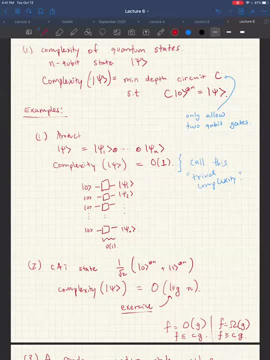 the most. What's the most general theory of nature that we have? Well, you know, I think a lot of people say the standard model of quantum field theory, or quantum. you know quantum physics And um, people have shown- at least you know, there are papers showing- that it's very possible. 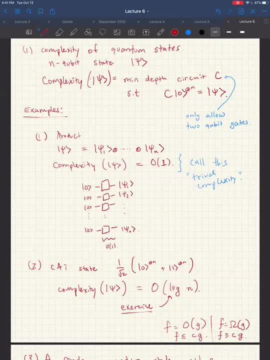 that you can simulate all of their algorithms for simulating the standard model in on a quantum computer. It's- it's not like fully proven, but it's. I mean it's it's. I think they have pretty compelling arguments for saying that here is an algorithm that can. 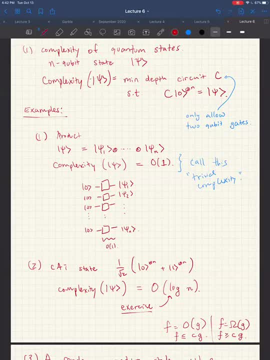 simulate, you know how all the fields interact and you know whatever in an efficient way, all in polynomial time. So, um, yeah, maybe I'll. I'll put send a link in the chat to this paper. There's a couple. 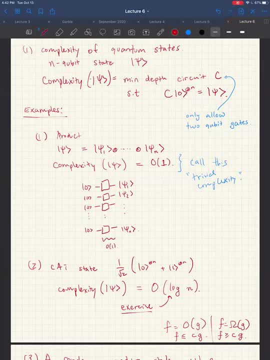 of papers that show how to do this. So if you think you know the universe is governed by the standard model, then then we believe you can simulate it in in quantum polynomial time. Hey, Henry, and just so. yeah, coming back to this, 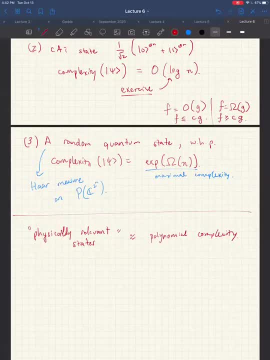 Yeah, Coming back to complexity theory, Uh, so we have, I mean, in the classical case we have, uh, you know, like a five end circuit, lower bound, right, But that's the best we have. So, um, what are some popular, I mean famous analogous uh cases for quantum circuits? 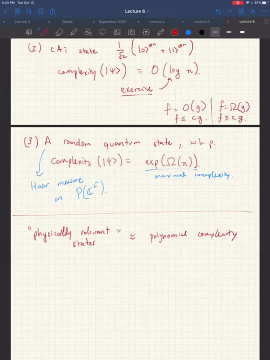 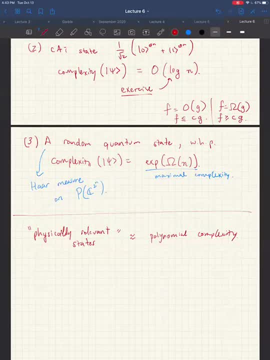 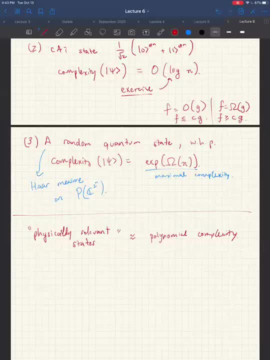 theory. we know even less in quantum complexity theory. Um, it's uh, I mean just to say, say some things like: um, for example, we don't even know the analog of a parody, not in. uh, it's an open question of whether a parody can be solved in quantum AC zero. 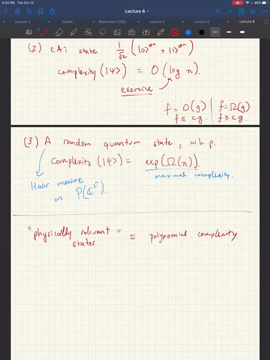 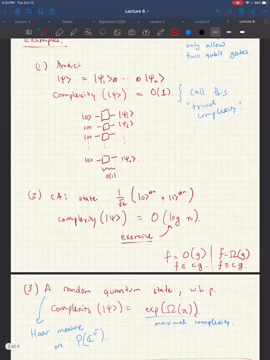 This is actually something that, like, Greg, has worked on. Yeah, So you know, we don't. we don't know that there's this thing with quantum state complexity, which I find very interesting because there's no, in some sense there's no- analog in the. so the analog of this quantum state complexity is this thing known as, like Kolmogorov complexity, which you might've heard of. 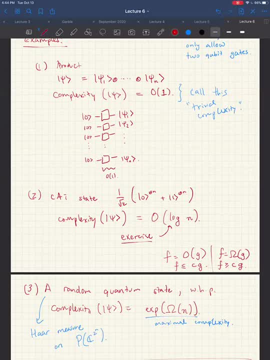 The Kolmogorov complexity. it's like it's a much limited range, Like it's it's a measure of how complex or how random a string is, And it is either between zero and n, whereas here it's between zero and exponential and n, So there's like a much bigger range for things to happen. 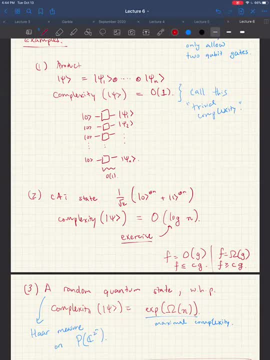 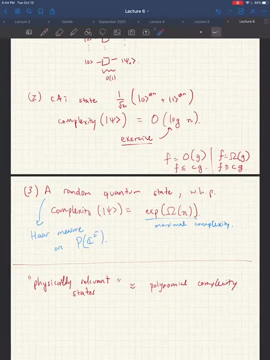 And one really interesting question I have is basically the only the best lower bound that we can explicitly prove on any family of states is this: one is a log n log Lower bound And it's a very- I mean. You can probably prove it yourself. 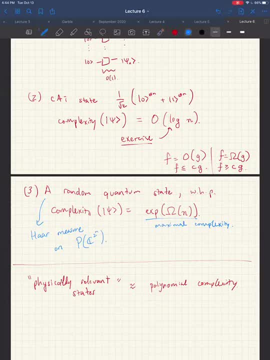 But one, one open question I think would be really interesting is: can you find a family of states for which there's a super logarithmic lower bound And, and as far as I can tell, there's no barriers to proving this, Like usually, you know, there's lots of complexity, barriers for things, but 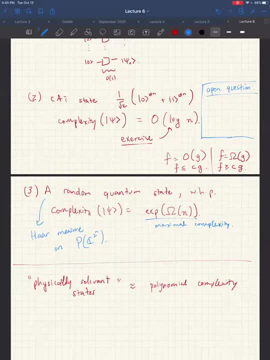 Yeah, But yeah, I mean, there's no barriers that I know of. Show you know family of states Such that the complexity Of Of this is is much, much bigger than log n, say, like log squared n. And do people have candidates for this? 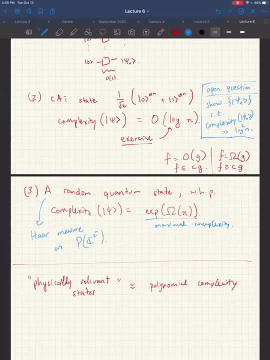 No, I don't think many people have thought about this. Oh yeah, It's like intuitively, why this is the case? because, like It's difficult to describe complex states, So I like to describe that these increasingly complex states would be, I guess, difficult to do. 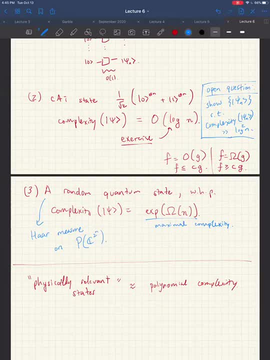 Yeah, you always run into problems like when you want to show something requires a large circuit to produce. you have to say there is no possible way of coming up with any simpler circuit. But our understanding of what's possible, what you can do with simple circuits, is we have a very- you know, we don't have a very good handle on that. 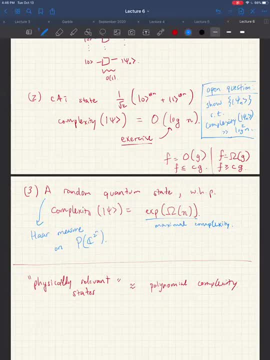 So you know, basically there's just like a lack of understanding, a lack of techniques, But also this it makes it like very exciting, because To me this is such a basic question. So again just a question: How do you prove that this is like the best possible scenario, like that's it? 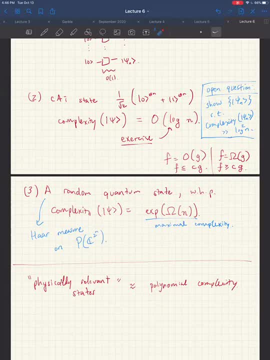 Because, again, we are not. we cannot produce all these states right for like it's a billion qubits or something like that, And you don't know if there is a Easier circuit or something like that. So how can we like, yeah, I can do, maybe like when, when you're thinking about moving these things, I can? 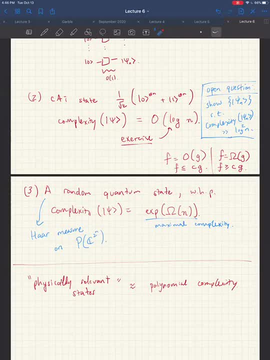 Like iteratively build up circuits and the best circuits for, let's say, 234 qubits. There might be some tricks here, but who knows what? what happens when you jump or bump up the number of qubits in the states, Right? So how can you like, like say that, that this is the best you can do? 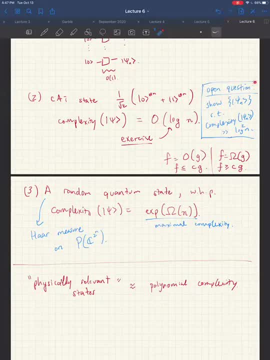 Yeah, that's a very good question. It's something that you know, The base, the basic answers. We have very, very few techniques for doing so like. let me just give a sketch of how do you argue this. So. so I said the exercises to prove that you can do it in login, But let me argue that you need at least login depth to do it and it's it's kind of. 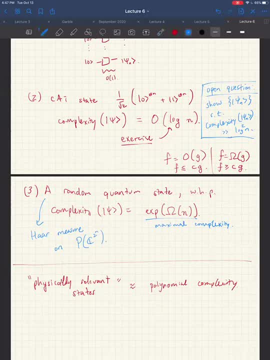 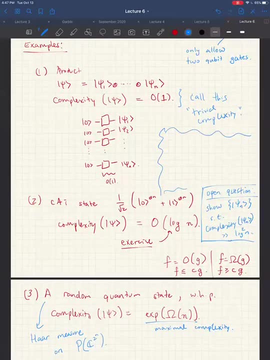 What? what's called a light cone argument Color should I use today? So Maybe, So let me try it here. So basically you say: well, imagine for contradiction that there was a circuit. Let's, let's even do something like kind of for simplicity, Let's imagine that there was like a depth 10 circuit that prepared the cat state, right, 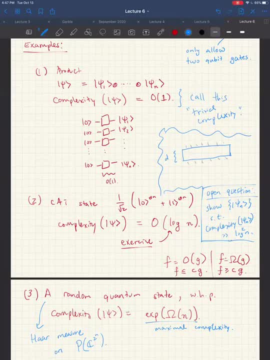 That started from You know All zeros And somehow produce the this cat state. Well, The observation is that you look at, you know, this output qubit here In some sense only can notice or did. it only depends on all the qubits in its past light cone, in the sense that if you, you know, if you sort of propagate, 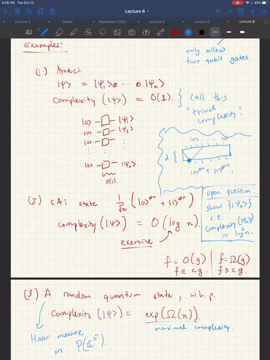 And I'm being very Wishy washy here, but you can actually make this formal, like the dependence of this qubit kit. It can only notice the the state of the input qubits that are connected to it. So there's that most. two to the D. 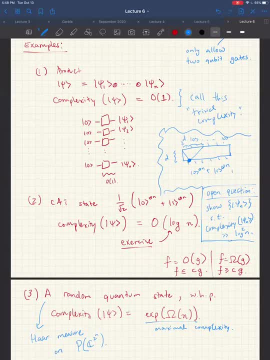 Input qubits that could possibly affect this output qubit. So that's not hard to show. but then And, and and- you know what you do- What you deduce is that if you can find a far away another output qubit that's far away, that has its own like home. that's disjoint. 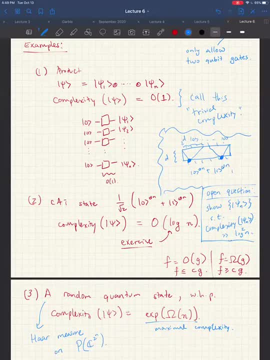 So it would. it would say that these two output qubits are behaving independently, But this cat in this cat state, That's definitely not the case. Like if you know that this first qubit is zero. Like if you measure this first output qubit and you get. 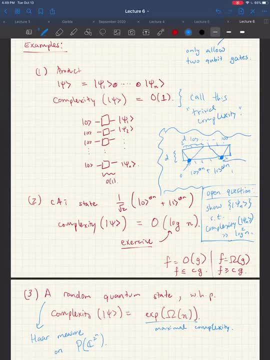 Outcome zero, Then you know that this output qubit also has to Be zero. Yeah Right, So so you know. so that that's sort of how you, you know, you argue that you can't have a circuit that's too short depth. 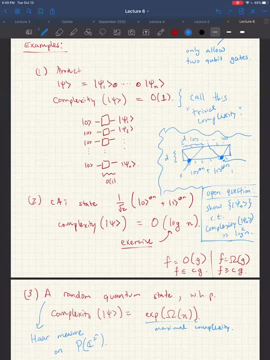 And, you know, embarrassingly, this is essentially the only technique that we have for proving quantum circuit lower bounds. And you can sort of see why we run to this log barrier, because you know, once D is log n, then this is Equal to n. 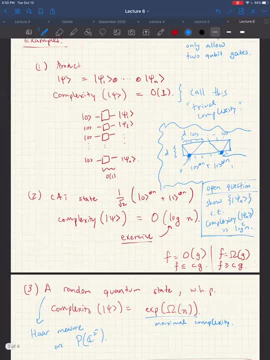 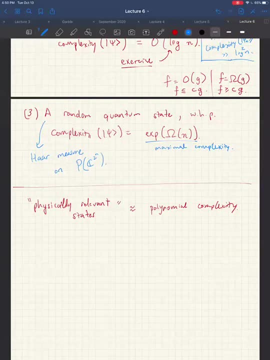 Yeah, okay, Thanks, Okay, Yeah, Great questions, So Okay. so we have this complexity measure and Let's let's come back to local Hamiltonians. You know there's. This measure motivates the following question: Which Local Hamiltonians? 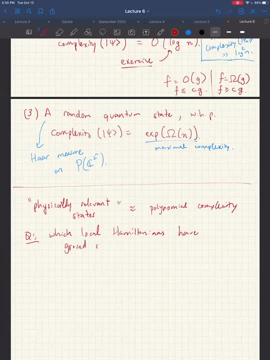 Have ground states Or, you know, low energy states for some definition of low With polynomial complexity. Okay, so this is a question you can ask And apply it to A potential answer that would be really interesting if this were true Would be, say, all physically relevant local Hamiltonians. 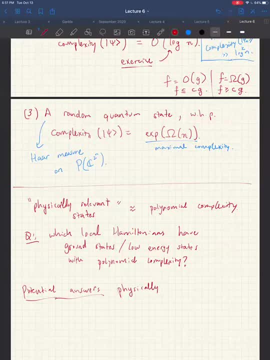 Physically relevant in the sense that you know it's the type of local Hamiltonian that you would encounter out in nature. If this were true, then that this would mean that you can always describe, you know, these physically relevant systems with polynomial size. classical descriptions there. classical descriptions because you can just describe the circuit that produces the state. 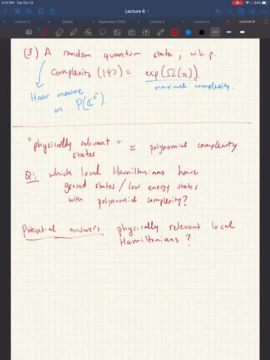 We don't know that This is true And it would be, you know, interesting either way. So we don't know, And but we can sort of just sort of think: well, what if you know? maybe we can define a complexity class that captures these types of local Hamiltonians. 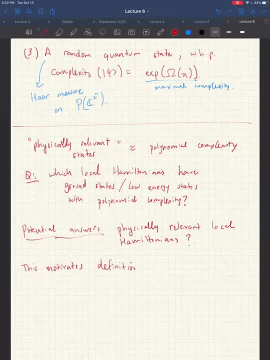 So there's this complexity class called- that's a variant of QMA Called QCMA. So this stands for quantum Classical and I personally think this is a horrible complexity class name, but people have just stuck with it. So QCMA and it's. it's actually horrible for a number of reasons. One is that it completely misrepresents what it means. 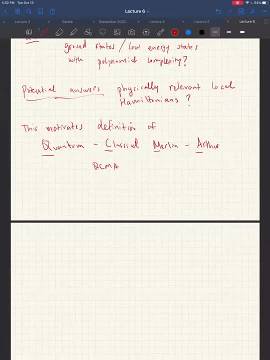 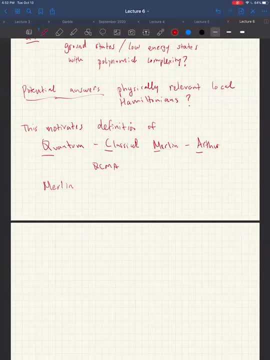 But Merlin can be used in a lot of different ways, So he can only send a classical proof. So Arthur is quantum polynomial time, And then Merlin is: You know, he's, he's, he's all wise and all powerful. but you can only send a classical string. 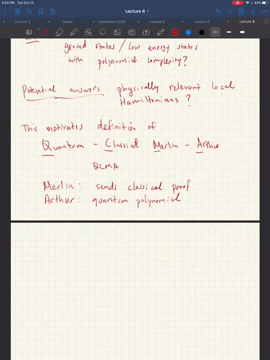 That Arthur verifies. Okay, So in particular, he can only send a classical string. So, in particular, he can only send a classical string, can only send a quantum state which is polynomial complexity. Yes, right, So this is sort of a more restricted version of QMA, and in terms of what decision? 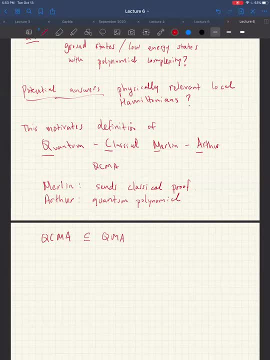 problems it contains. well, it's going to be a subset of QMA. We don't know if they're the same or not, but I mean the question of whether they're the same is really like the. it sort of captures this question right here, Like if they. 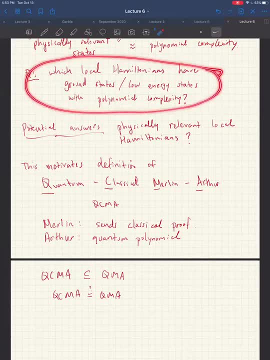 were the same, then it would say that essentially you can always describe the you know ground states. you can always give like a classical proof of a ground state. you know a classical proof that a local Hamiltonian has a low energy state. 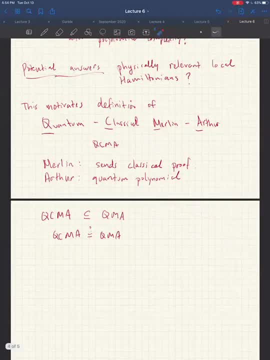 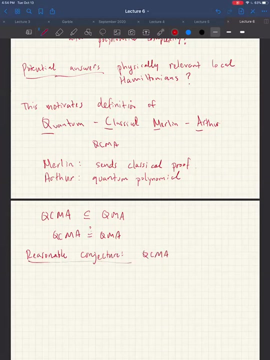 Yeah, And then a reasonable conjecture- well, reasonable to some people- is that they're different, That actually the ability for Merlin to send you a quantum state to convince you of something is actually a powerful ability. Okay, So this would imply that not all local Hamiltonians have polynomial complexity ground states. 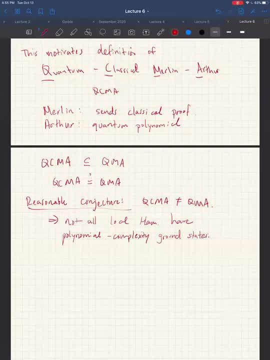 Okay, So let's connect this to the quantum PCP conjecture. So QPCP plus the assumption that QCMA is different from QMA would imply that not only do ground states in general don't have polynomial complexity, but even, if you consider states that have much higher energies, right? 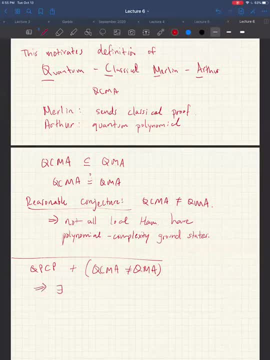 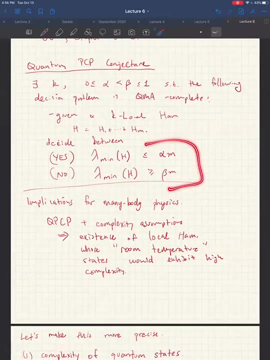 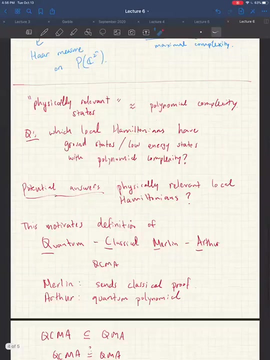 up to this medium energy range. Okay, So it implies that there are local Hamiltonians whose states with energy less than beta m, where this beta m is this, you know, threshold between yes and no, right this: that any states that have energy less than this cannot have polynomial complexity. 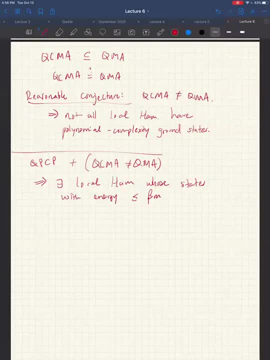 Okay, Okay, Okay, Okay. Oh, I thought What happened. Okay, Okay, Sorry, I'm working. Sorry, Sorry, Yeah, Okay, All right, we're getting this just back to normal data type, Perfect, Okay. 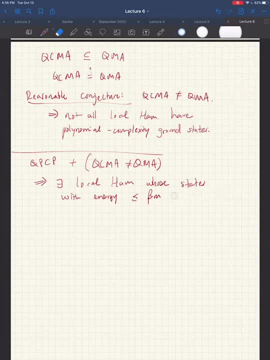 Okay, All right, so they're not including and not infhee- sunny, I'll have a. I'll have superpolynomial complexity, All right, okay, Perfect, Perfect, Perfect, Alright, great, It will Super Super. 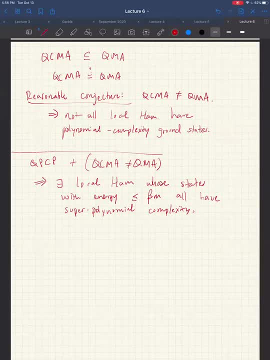 Super. Okay, all right, Super. So this is super, Super. you know, getting closer to, or this is a more precise way of stating what this many-body physics implication of the quantum PCP conjecture would be, And you. 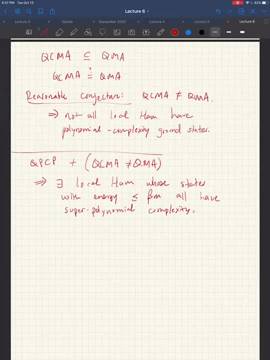 know, what does this have to do with temperature, right? I was saying like room temperature, right? And again, you know, there's this loose connection between energy and temperature. We can actually make this a little more precise, and I kind of alluded to this last time. 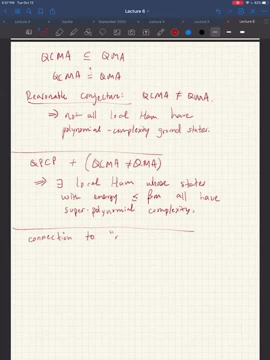 So what's the connection to room temperature? So you know, remember that a local Hamiltonian describes a physical system like what are the forces at play, the interactions, the constraint of some physical system. So here's a local Hamiltonian, Here's a system S with a bunch of particles, right, You know some? 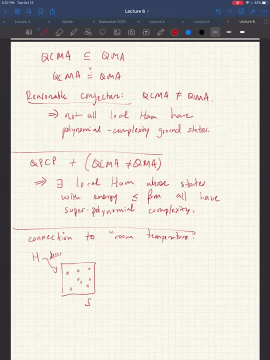 cubits. So this Hamiltonian describes the interactions right And depending on the configuration of your particles that you know, your system would have different energies. Let's imagine that. and okay, I'm going to start to get into territory that I'm kind of a novice in, but you know people who know better. help me out. So 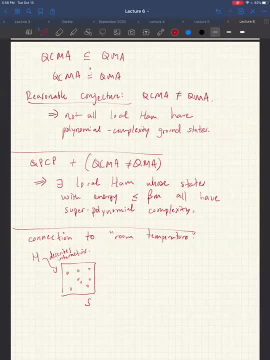 when you have the system and you put it into contact with an external environment, right? So I'm gonna put it in contact with something known as a bath that's much, much bigger than the system S right, And this bath has you know. 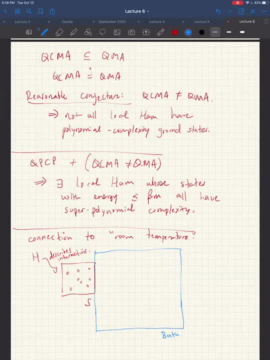 you can think of it as having an infinite number of particles and it's like in equilibrium And it's. you know there's some interactions between these two And you know this bath is at some temperature T And if you sort of let these two systems interact, 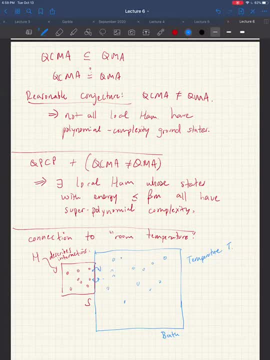 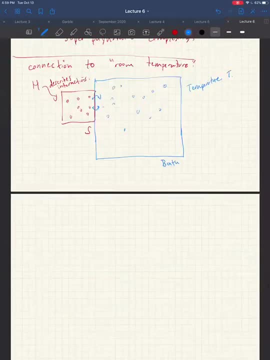 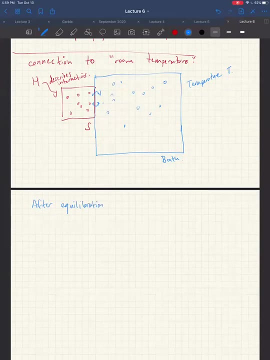 and equilibrate. eventually, both systems will be in temperature T And then you can ask: well, what is the state of the system S? And it's going to be in something known as a Gibbs state. So it represents the state of the system. 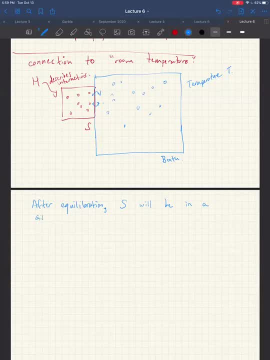 at thermal equilibrium. And what is this Gibbs state? Well, I'm gonna denote it. It's a function of the Hamiltonian and the temperature And it's the following density matrix: it's going to be 1 over z and it's going to be e to the minus h over t. And what is z? 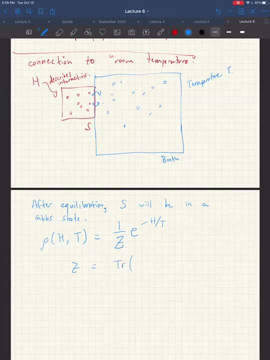 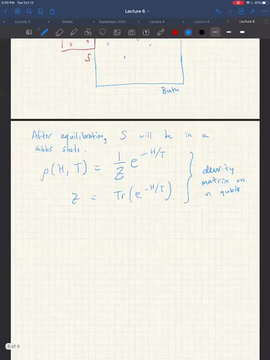 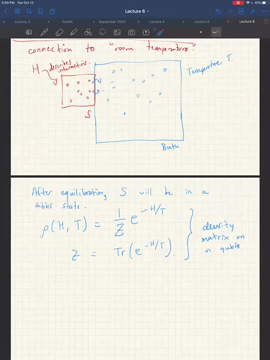 It's the normalization constant, It's the trace of this operator, So you can verify for yourself that this is a density matrix. It represents a probabilistic mixture of pure states. It's a density matrix on n qubits And it's supposed to represent the distribution of states of the system S. 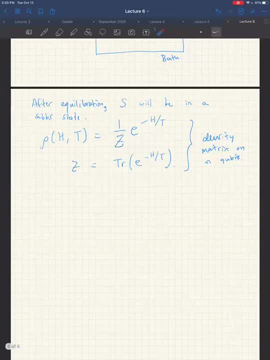 So what are some features of this Gibbs state? So here's where we can connect things to what I said. The minimum eigenvalue is like absolute zero and we can make that formula. So as you drive the temperature down to zero, then this Gibbs state approaches. 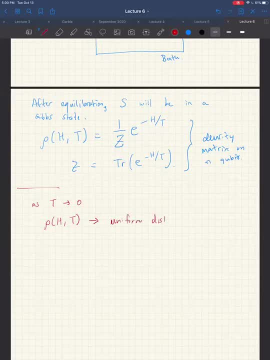 the uniform distribution over the ground space of your Hamiltonian. So it's really just going to be the just an equal mixture of ground states. So it's really kind of tells you that if the temperature of this bathroom is going to absolute zero, then really that's going to cool your system down to the ground state. 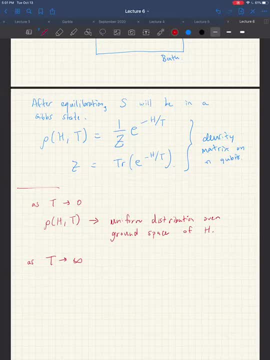 On the other hand, if you're going to crank up the temperature to make things hotter and hotter, then your Gibbs state is actually going to approach what's called the maximally mixed state. So it's 2 to the minus n times the identity. So this is a density matrix. This is the maximum. 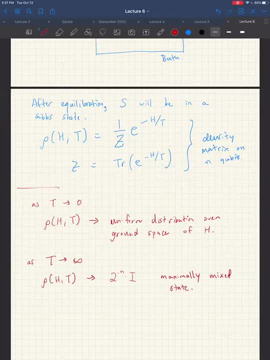 mixed state. And let me emphasize, it's the maximally mixed state as opposed to the maximally entangled state. In fact, the state has no entanglement whatsoever, It's completely featureless. I mean, this state just looks like the uniform distribution over all- classical bit. 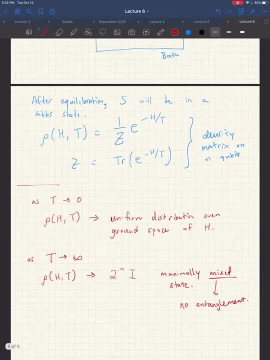 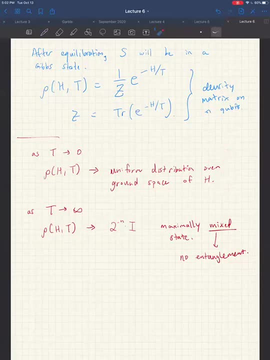 strings Right. so if we took a Hamiltonian that you know had a complicated ground state at ground zero but then you cranked up the temperature, it's going to lose all of its quantum effects as things go to, as the temperature goes to infinity. 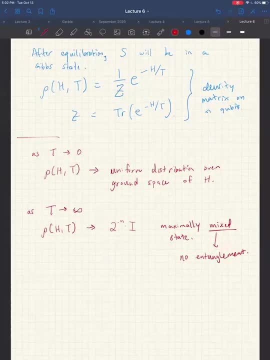 So, you know, given this, given like a Hamiltonian, you can ask: well, what's the crossover point between when the Gibbs state has, you know, high complexity and to when it has low complexity? right, There's a certain temperature at which, there, you know, 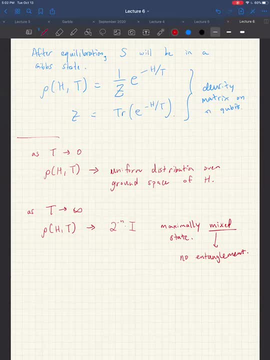 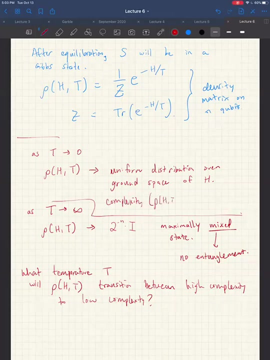 there's some transition point, Right, so actually let me so here. the complexity of this mixed state- and what I mean by this is that you know it's a mixture of you know what's like the average complexity of all the 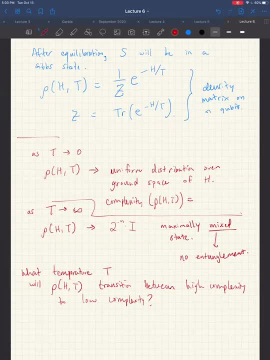 states in its mixture. It's going to be, you know, very large, say super polynomial, But here the complexity of this maximum mixed state is going to be zero, or, you know, order one. So it went from very large to order one. and what's the? at what point does it switch over? 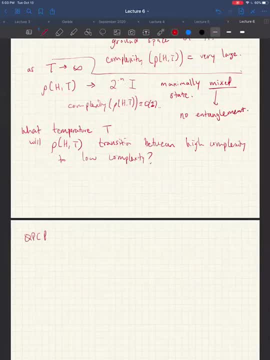 Okay, and so what the quantum PCP conjecture says? you know, quantum PCP plus QMA not equals to QCMA. it implies there exists local Hamiltonians where this, where the complexity of this Gibbs state remains high, even when 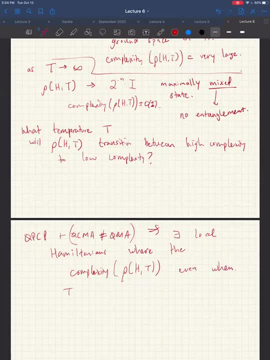 even when the temperature is, is some growing function of the number of particles. Okay, Okay, And so? so this is really how you can make this, this claim that it's saying something about, you know, room temperature entanglement. You can make this statement precise. 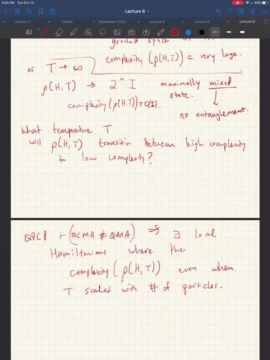 And and actually in the, in the next problem set you'll, you'll make all of these statements more precise and quantitative. So, like you're assuming that there's some threshold phenomena here, I guess there's not necessarily a threshold phenomenon. I guess I want to say what's the point at which it switches from? 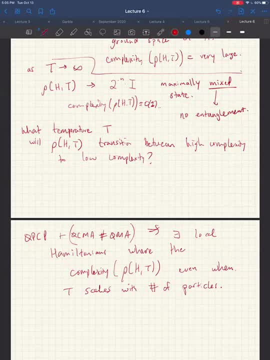 you know we're, we're also talking, you know asymptotically right, But is there a point at which it switches from super polynomial to polynomial? Okay Yeah, Henry, is it known that I guess, if QPCP and QCMA is not equal to QMA, then the same local Hamiltonian H works for? 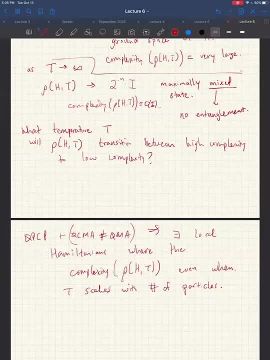 for both implications or could they possibly be different? You mean for QPCP and QCMA not equal to QMA, Right? So I guess you have two different implications, but I guess I are they going to be equal to the same local Hamiltonian H. 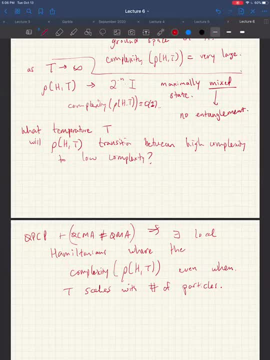 Right, So I guess you have two different implications. but I guess are they going to be equal to QPCP and QCMA, not equal to QMA? they are they known to imply each other? oh, you mean the what I wrote before like 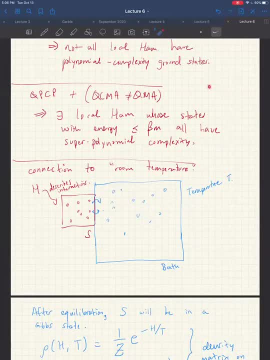 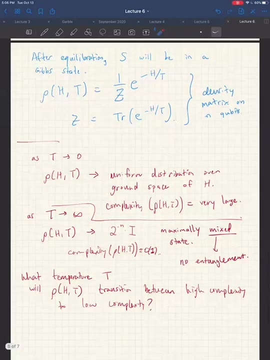 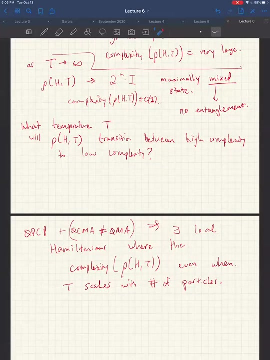 like this one right, and the Gibbs state one: oh, they're, they're roughly equivalent and actually this is the equivalence, is what you'll like, proven the the problem set. I guess that that kind of makes sense. yeah, okay, so let's take a five minute break. so let's come back at, like you know, 511 ish. but you know we can. 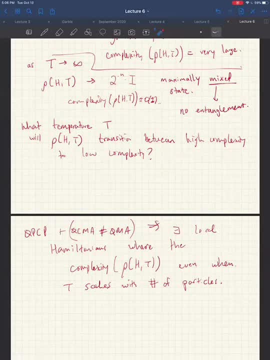 continue chatting. people have more questions. so, Henry, I just found the paper that was trying to recall. I can post it in the chat. okay, so I'm not quite familiar with the with the work, but I know well, I knew that that input a very well and it seems to say: 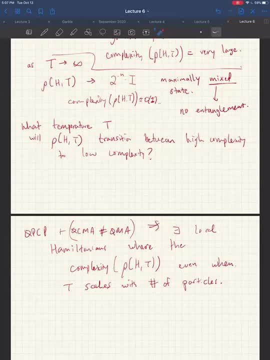 that that most states in the Hilbert space are not physical, because they looked at which states could be prepared with a time evolution under a local Hamiltonian or time dependent local Hamiltonian in polynomial time, and they found out that this set of of states is occupies only a exponentially small fraction of the total Hilbert space. 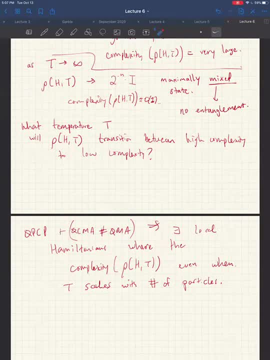 so I think that's a that's an important reason there which kind of corroborates what you were saying. I just need to get past the paywall. I can also share this with you if you have any other questions. if you have any other questions, please feel free to put them in the Q&A box below. 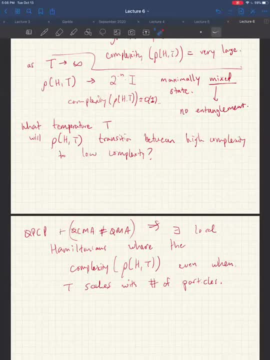 I can also share this with you if you have any other questions. if you have any other questions, I can also share this with you if you have any other questions, if you have any other questions, and I want to share that PDF as on Slack, I guess, Oh sure. 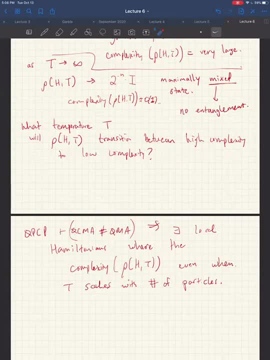 Yeah, I think I think this is basically in the same spirit of what I'm saying, But I would imagine that they didn't actually identify, they didn't pin down any specific states that would require an exponential amount of time to produce. so you know that. you know that if you just sort of close your eyes and just 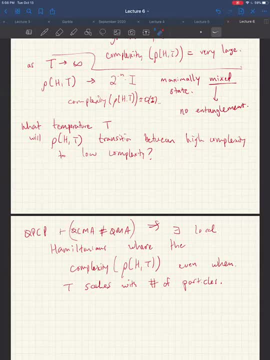 reached out and grabbed a quantum state at random. with high probability it's going to be exponentially complex. But to actually guarantee to me that a state has exponential complexity, this is something we don't know how to do, Right? Yeah, And also, you can think of someone before quantum computers and you ask them. okay. 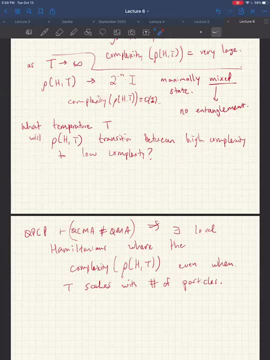 is it possible to store a 200 qubit state? They say no, that's impossible. I mean we don't have the technology to do that or whatever. but then today's possible. So but it's hard to prove that there is no technology that we don't know that can prepare. 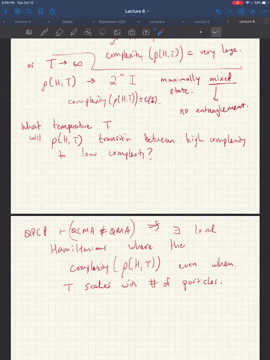 in polynomial amount of time and state Right. My power went out for a second. I'm going to take a few minutes at physically relevant states. Oh no, So did I miss anything important? Well, the good thing is that this video is recorded. 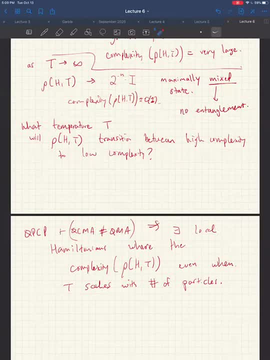 So that was quite some time ago, right, Like that was like half an hour ago or something, I think like 10 minutes, 10 minutes ago or something. Okay, I think we were just mostly chatting, But yeah, everything will be recorded. 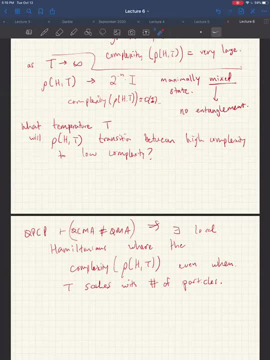 So Okay, Cool, You can review. Oh yeah, I don't think last week's recording is out yet, Is it not? I thought they posted it. Did they post it? I think it was posted in the Slack, Oh okay. 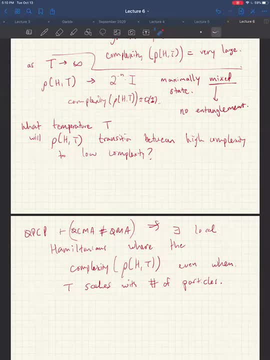 Like like a week ago almost. Let's see. Yeah, It's a video of lecture five, So so if you have access to the Slack, you should be able to see it. All right, Thanks, Can you please repeat the last sentence that you wrote there? 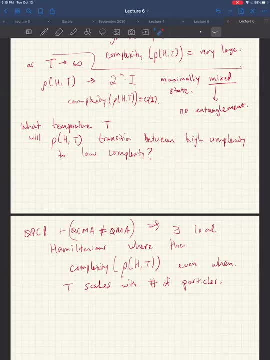 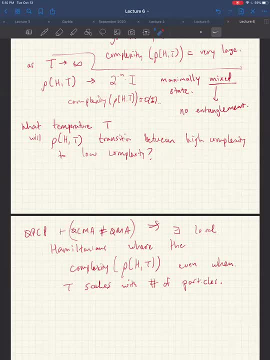 even when T-scales with number of particles are. I feel like there's a word missing there somewhere or I'm not understanding it. Oh, were the complexity. Yeah yeah, Complexity is super polynomial. Okay, Yeah, Right, All right. 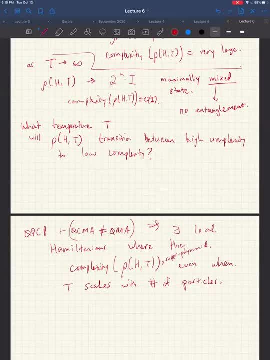 Okay, Okay, Okay, Yeah, I wanted to ask. so what restrictions of quantum circuits have been studied? I mean, again, comparing it to the classical case, you study, of course you study bounded depth quantum circuits, but apart from that, I mean you study monotone classical circuits. 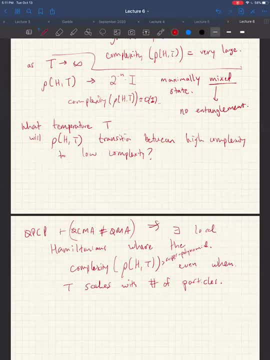 you study, let's say, formulas, right? So have people looked into proving lower bounds for maybe restricted settings of quantum circuits? Very little, I think we just don't have enough interesting classes of restricted, restricted classes of circuits that are amenable for analysis, but I don't know. 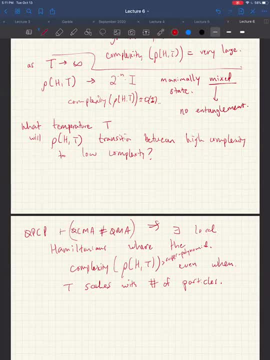 People think about, yeah right, constant depth. I think people think a lot about circuits where the connectivity between the like the qubits are all arranged in like a grid, or in some, you know there's some like limited connectivity, I mean because that's motivated by activity. 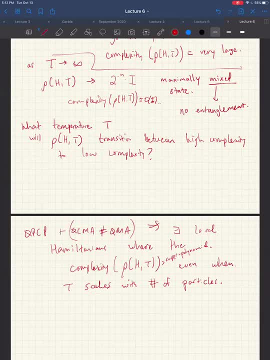 We're actually trying to build these computers. in terms of other restrictions, How would you define a monotone quantum circuit? What does it mean? That's a good question, I don't know. I mean. what about the formula, though? What formula? 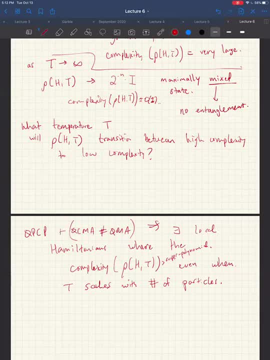 So formulas, So remind me, Formulas are where you cannot repeat input bits, right, Yeah, So So the underlying tree is acyclic? yeah, Right, So I guess with quantum circuits, you, you're not allowed to copy quantum. you know quantum. 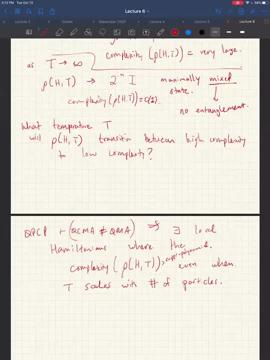 bits anyways. So, Yeah, That's a good question, I don't know. Yeah, Yeah, I don't know. Or I guess, equivalently, formulas are just locked, locked up circuits. Yeah, So you know. so the the, the notion of, there's this model of quantum AC zero which is supposed 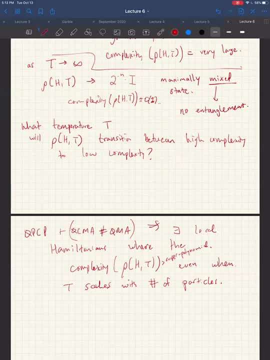 to be the quantum analog of classical AC zero. and there they. you know it's. it's like the standard model where you have two cubit gates, but they also throw in these really long range gates called quantum fan out, Which allows you to copy input bits. 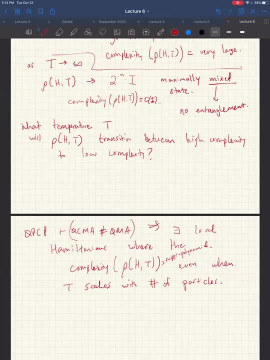 Sorry, I okay, Let me back up. There's there's two notions of quantum AC zero: one with or without fan out, And and. and this is sort of like the big question: Are they the same with fan out? 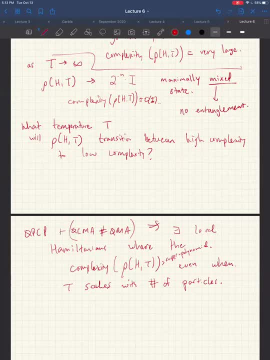 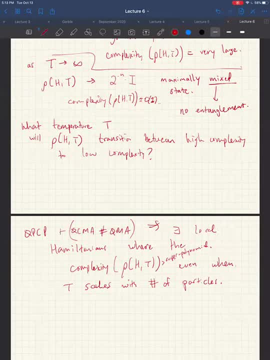 Yeah, Yeah, Yeah, Yeah, Yeah Yeah, Leaving this fan out gate, which is very curious. And so the question is: well, if you don't have this fan out gate, can but you have these other types of long range gates, can you still solve parity? It's, it's not known. So what do you mean? what long range gate? Oh gates that act on like a growing number of cubits assignment all at once, like you know, like a square root and sized gate or something. 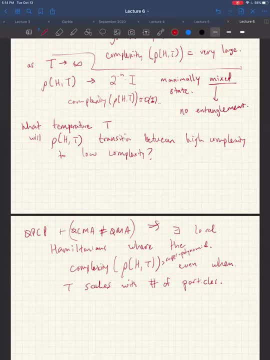 I guess in the AC0 model your fan-in is unlimited. anyway, Yes, right, Right, right, right, yeah. I guess it's interesting because I think you mentioned, Henry, that like people in like experimentalists, are implementing these like fan-out gates or something like that. 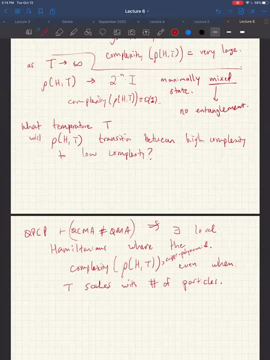 Yeah, so there was a paper that came out a month or two ago that said on, like ion traps, that you can actually do quantum fan-out, which might mean you can solve parity in constant depth circuits, quantum circuits, Which would be pretty cool. 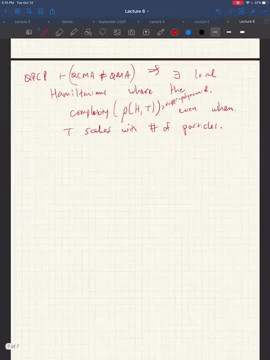 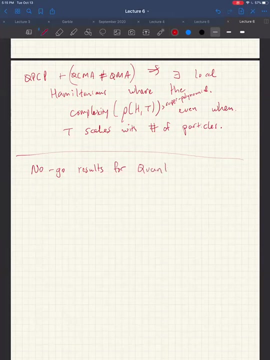 Okay, so let's get back to it. Let's see all my notes. Okay, so I want to talk about some no-go results And basically this is. you know, I've stated this quantum PCP conjecture. A lot of people find it very interesting. 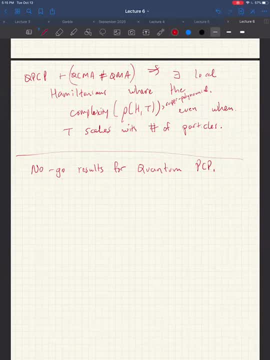 So what's known about it? Not a lot. Basically, the best things we know is: if you were to try to prove quantum PCP, here's what you should do. That's basically what people know, So I'll cover them. One is: quantum PCP cannot hold for local Hamiltonians defined on a grid. 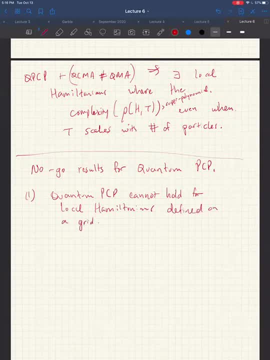 Okay, so what do I mean by this? Well, quantum PCP is saying that you know, we're restricted to local Hamiltonians where you can encode QMA-hard problems into them, And it's QMA-hard even to tell whether they have like really really high ground energy or really really low ground energy. 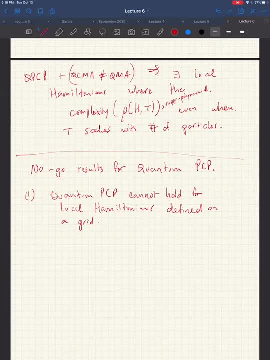 So, ultimately, if you were to say, prove the quantum PCP theorem, you're going to construct a really exotic family of local Hamiltonians, Just like you know, when we constructed this Cook-Levin theorem, This Feynman-Kataev Hamiltonian had. you know it has some qualities, right. 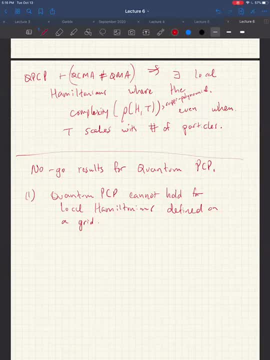 Like it's. you know it has like these, you know these clock qubits and it has these like starts okay, evolves okay, ends okay terms and so on. right, So you've constructed some family of Hamiltonians. Quantum PCP requires some other construction. 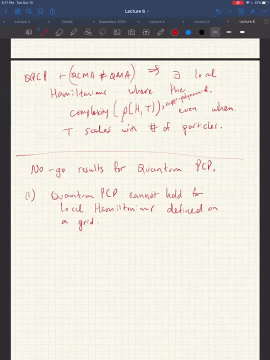 But what we know is that your local Hamiltonians cannot- Cannot- have constraints that lie on a grid. So what I mean by this is that you can't have a Hamiltonian where you have qubits in, say, some 2D grid. 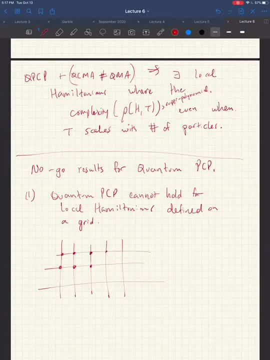 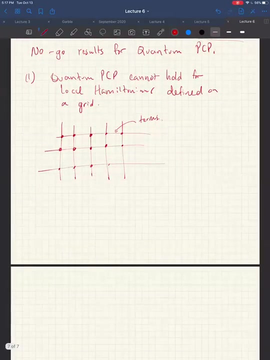 Say: qubits are all in the corners here, And then all the Hamiltonian terms act on nearest neighbors. And why is that the case? Well, the point is, if you had a local Hamiltonian of this form, so let's say it's. 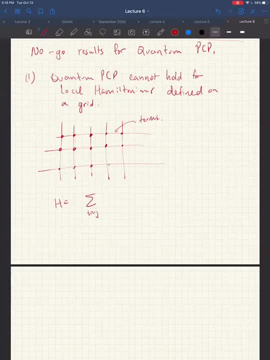 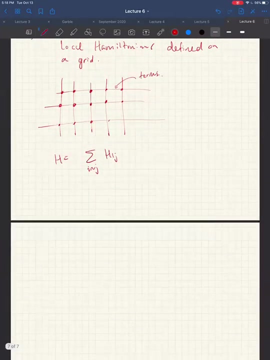 If qubit i is connected to qubit j, then you have a term connecting them. If you had a Hamiltonian of this form, then in fact you can always approximate the ground state using a product state, Right? So actually there's just very, very little entanglement needed to describe a low energy state. 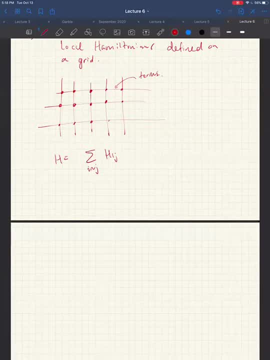 And that would mean that you know you can always give like a classical description. But if you're assuming this thing, that you know QMA hard problems can't have efficient classical descriptions, then this would be a contradiction. So basically, what I'm going to show is that 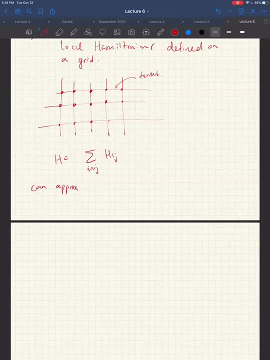 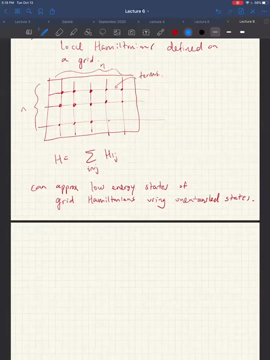 You can approximate. So the way we're going to do this is So. let's say that our grid was n qubits by n qubits, So there's n squared qubits total, And we're going to chop up the grid into little L by L patches. 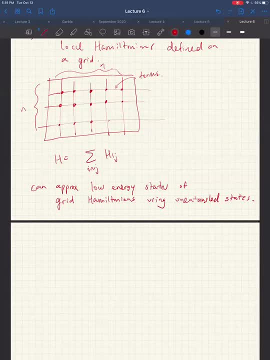 So Or L by L, patches Or blocks, Right? So we can say, Let's block together these L qubits, Right? And then you know, we just put the blocks together like this. So let me just tile them. 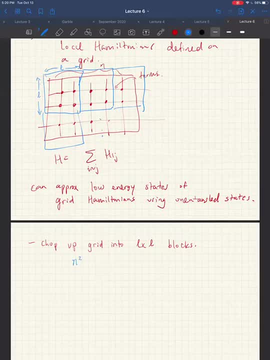 And so ultimately, we're going to get N squared divided by L squared, L squared, blocks Right And within a block we can. You know, there's a bunch of Hamiltonian terms And we can group the Hamiltonian terms together. 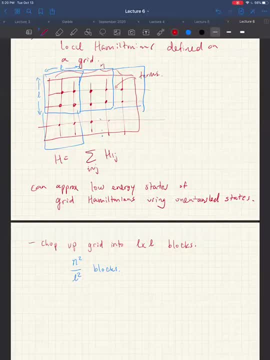 So let's see How should I? So let's label each block. You know one through N, squared over N squared over L squared, And I'm going to define a new Hamiltonian term for the ith block. So this is going to be the sum over all say qubits. 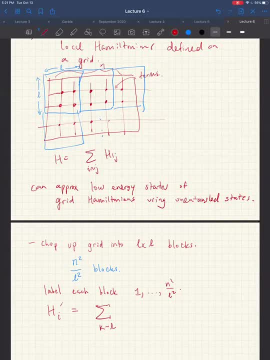 Qubit K is connected to qubit L And both are K and L Are in the ith block, Right. So you're going to look in a block and you're just going to look which Hamiltonian terms go between qubits that are within the block. 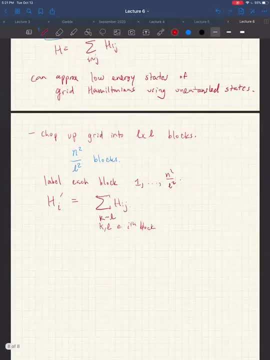 And we're just going to include those. Okay, So I'm going to call this H. I prime a super term Right, So super Hamiltonian term. You just sort of cluster them together And I'll define a new Hamiltonian that I call. 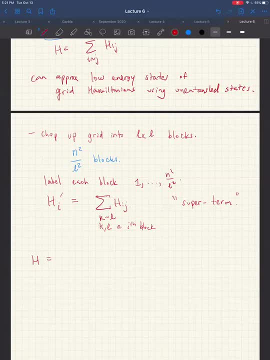 Well, actually, Let me say, The original Hamiltonian H can be written as a sum of these super terms. So let me call this M Right. There's M blocks, Right, But we've omitted some terms Right, Namely the terms that go in between the blocks. 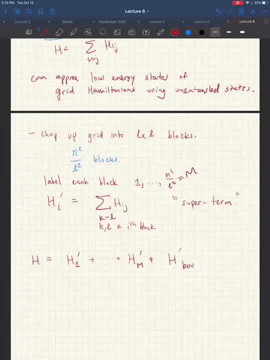 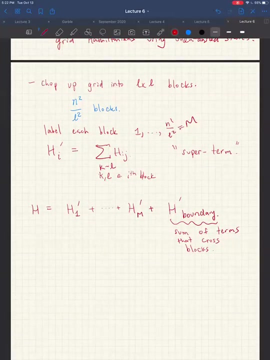 So I'll just call those the boundary terms And I'll just bundle them all together into another super term called H boundary. Does that make sense What I'm doing? Okay, Let's first just do a quick count of how many boundary terms there are. 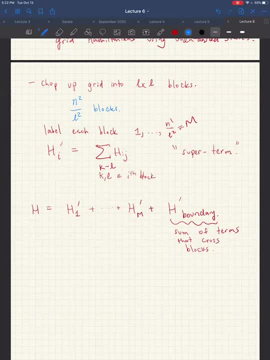 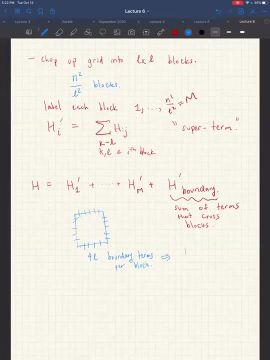 So each block has roughly four L boundary terms Right And there's N squared over L squared blocks. So in total there are four N squared over L boundary terms Divided by two. maybe Divided by two, Oh yeah. 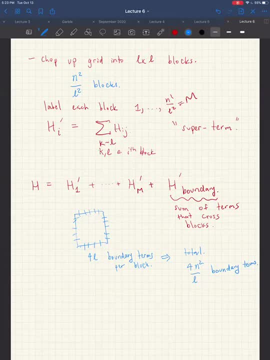 Probably Because you're double counting or something, Right, Yeah? So let's say at most, And that's four N squared over L boundary terms, All right, Okay. So let's look at a super term. Okay, Let's just call it H. 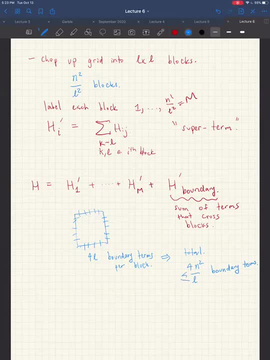 Okay, So let's just call it H. Okay, So, let's just call it H. Okay, Okay, So, let's just call it H. Okay, Let's just call it H. Okay, Okay, Okay, Okay, Okay. 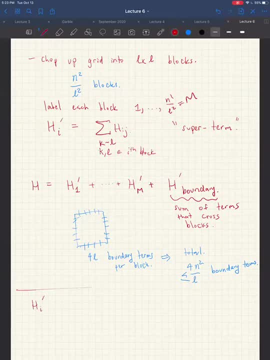 All right, So let's call this term H prime I All right, It's a by itself. this is like a mini local Hamiltonian that acts on L squared qubits. Okay, And let's think of L as just being some large enough constant like 100.. 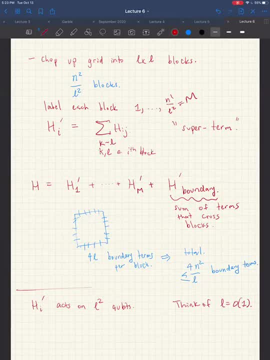 Okay, So it's just some constant. It's not growing with the size of your grid. Okay, And the ground state of this mini Hamiltonian can be found in 2 to the L squared time. You just brute force this little patch and solve for the ground state. 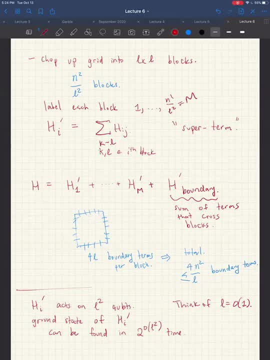 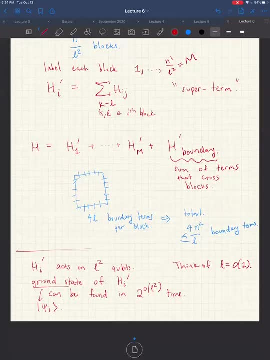 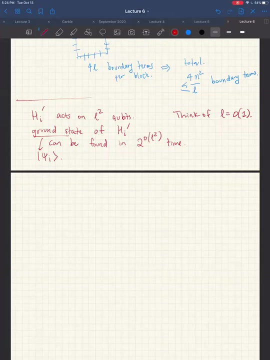 So let's call a ground state, psi, sub i. So for each of these blocks we're going to individually solve for those ground states and then we'll just piece them together, And so we'll just say: I'm going to define a state, that's going to be my approximation. 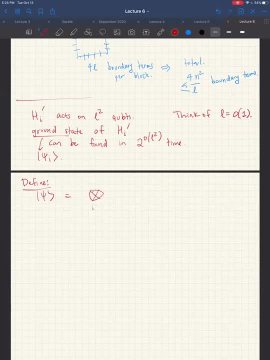 of the global ground state as the tensor product. Okay, So this is going to be my approximation of, you know, patch 1 up to patch n, squared over L squared of psi i. So this whole state is going to be on n squared qubits, right. 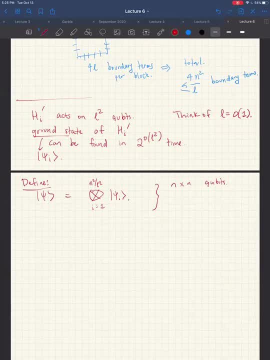 It's on n by n qubits, But since it's this product state, it's going to have a very succinct description, right? I can describe it just using, you know, just by describing each of the psi i's individually, right? 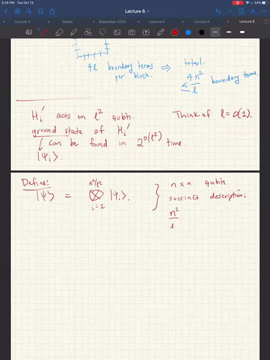 It can be described in. you know the number of patches times the size of each, the description size of each ground state individually, And you know this is still. if L is a constant, then this is still polynomial of n, right? 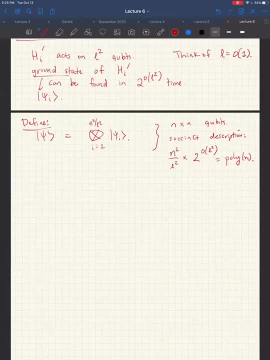 And now let's compute its energy and let's show that it actually has a pretty low energy. Okay, Just one quick thing. When you say brute force on h i prime, you mean like take the matrix and and and compute its and and its and compute its e, e in vector corresponding to its smallest e in. 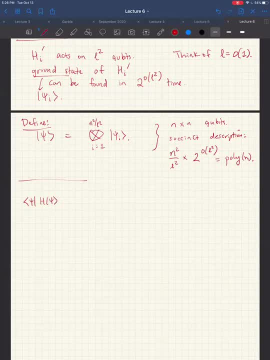 value. Okay, Yeah, That, or you know, that's one possible way to do it, Okay, So let's, let's expand out what this is. Let's first sum over all the patches. So we're going to have a psi, inner product patch i, and then we we have, you know, these. 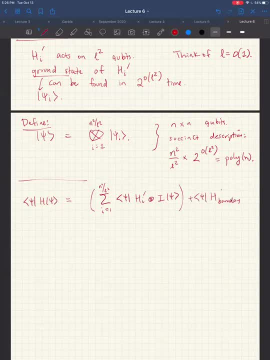 boundary terms right. So here we. since this is identity on all but L squared qubits, we can actually just- and this size is a is a tensor product of states. We can just isolate the i-th ground state. 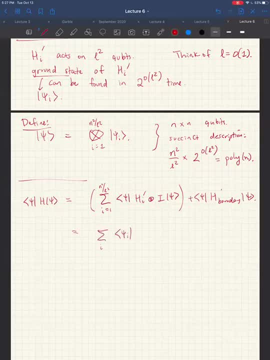 So this is just equal to sum of mission over: i psi i, h, i, prime psi i. And then we still have this boundary component right Here. I'm just going to, I'm going to upper bound this just by the norm of this Hamiltonian, this, these all. 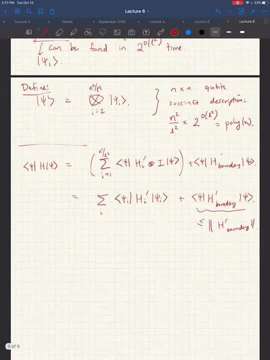 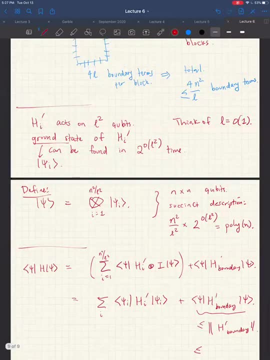 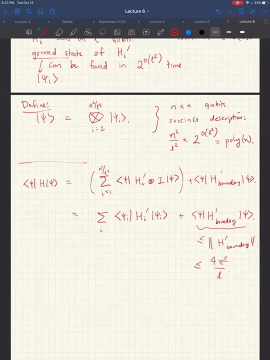 these boundary terms and you know, basically we can just upper, bound this by counting the number of terms that are present, and how many terms are there? Well, that's the number of boundary terms. We've calculated this to be a four N squared over L, some or some constant N squared over. 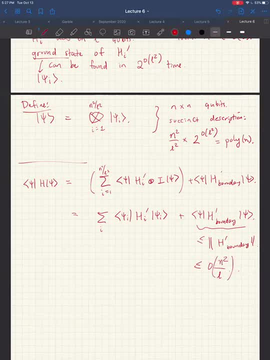 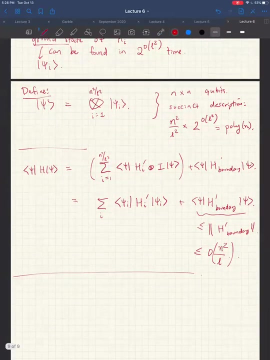 L. Okay, So we can just do this. Okay, Everyone following so far. So now we just have to see how well. I mean we want to relate this to the minimum eigenvalue of H, right? So let's do another calculation, which is: let's take the actual ground state of H. 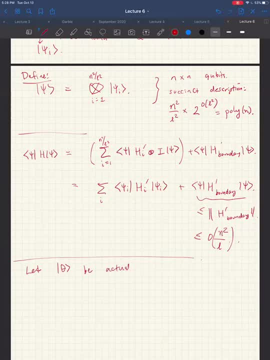 So let's let theta be actual ground state of H, Okay, Okay, And this is our initial ground state of H. So we know that lambda min of H is going to be the energy of theta and this is going to be at least- again we're going to sum over these super terms- we have theta, HI, prime. 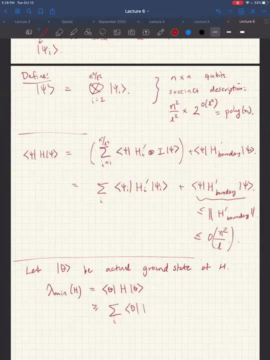 theta H, I prime, Okay. And then we also take this and subtract it, Okay. So we have theta H- I prime, theta H I prime, theta H I prime. So we've got this. these are the two super terms here. 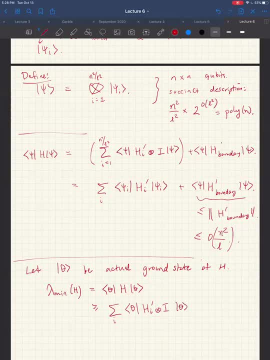 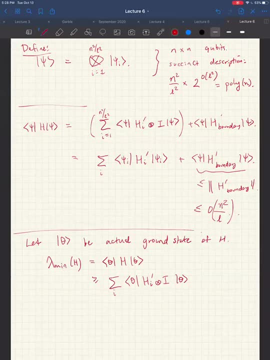 Okay, This is the first of the super terms, theta, and we actually can just drop the boundary term, because that's always. you know, the energy of theta with respect to the boundary terms is always non-negative, So we can just ignore it. 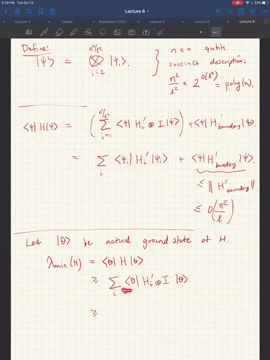 But now we claim that each of these we're trying to here minimize, you know okay, the energy of theta with respect to this super term, hi is always going to be at least the thing that we already found to minimize it. 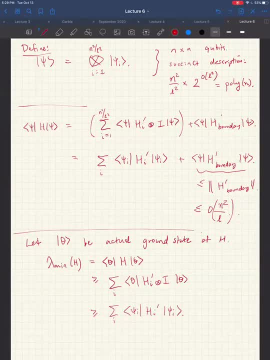 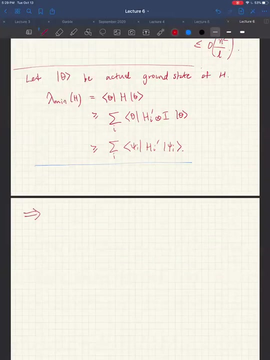 Okay, So basically we can now just combine these two derivations, and what do we get? We get that the energy of these block states is going to be, at most, the minimum eigenvalue of H, plus this error term, which is four N squared over L. 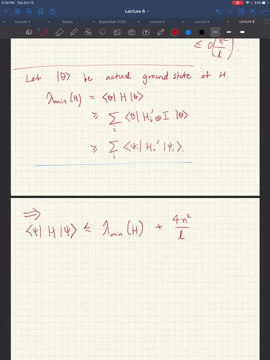 So we're only doing worse than the minimum energy by this, by this additive factor four N squared over L. Let me normalize this to be more in line with how we've been talking about the quantum PCP theorem, Like we're talking about the, you know. 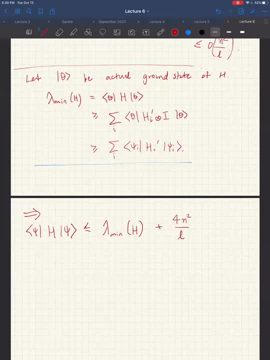 beta M or alpha M, where M is the number of terms. So you know the number of terms is going to be, you know, order N squared. So if we do the substitution, we see that really this, this error term, is the number of terms divided by this L. 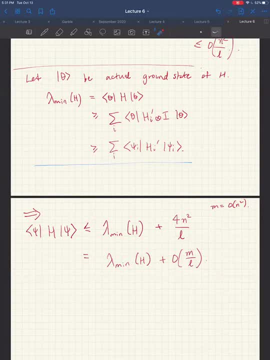 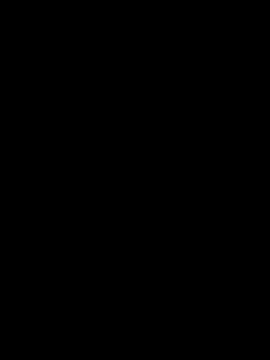 which is, you know, some, some large constant, Okay, So you know, suppose that. okay, how does this tie into? sorry, So let's say that Your screen stopped sharing. Oh, it is stopped sharing. Oh, let's see. 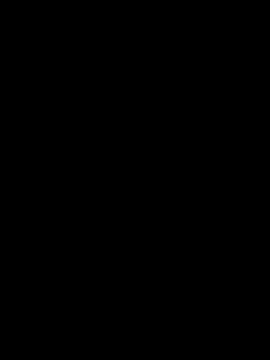 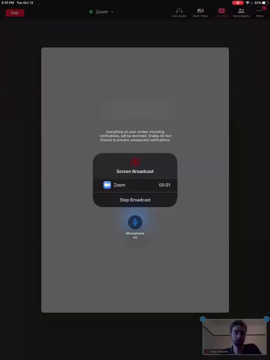 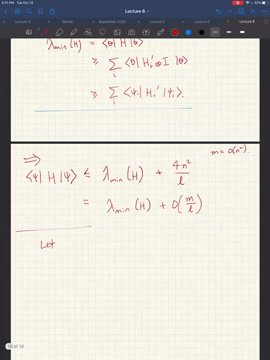 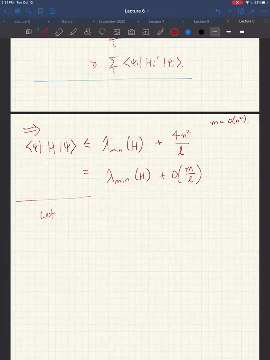 What do you see? now I'll start broadcast. Okay, Are we back? Yep, Okay, Awesome, Thanks, Okay, So so coming back to like you know. so why is this a no go result for quantum PCP? 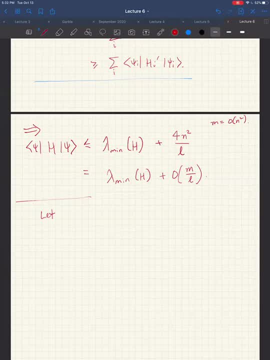 Well, the point is that here's a ground, here's a state for H that only has, you know, M over L, extra energy above the ground energy, And it has a very succinct classical description. And, if you know, M over L, extra energy above it. 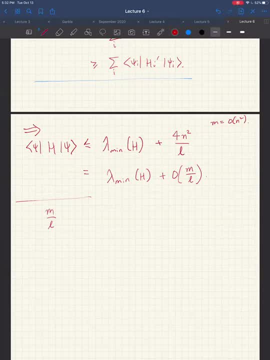 uh m over l is, you know, much, much smaller than the difference between uh beta minus alpha m. then you know, then we're technically in the, the yes case, right, because, um, you know, the, it means that the the minimum, um, the minimum. i can you know the ground energy of this local hamiltonian? 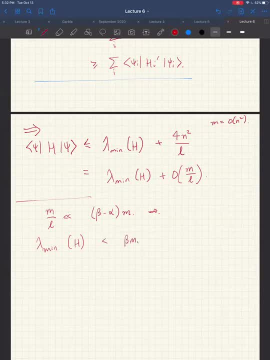 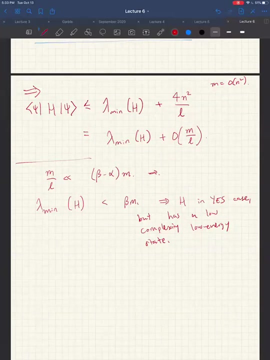 is going to be, uh, much smaller than than beta times m, so which means h is in the yes case but has a low complexity, low energy state. okay, so does that make sense to people? okay, and you know, there's nothing special about 2d grids in this argument. this could. 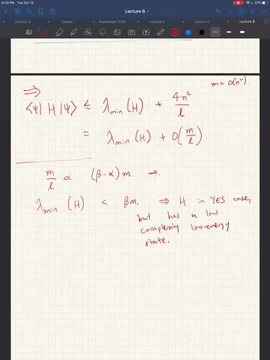 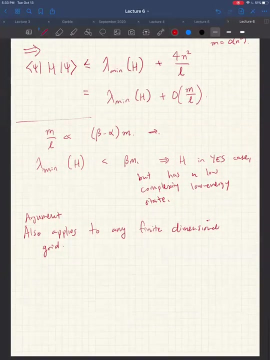 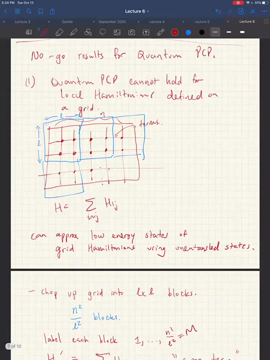 have applied to any finite dimensional grid, um. but so the general question is: why is this so important? so the you know the argument, um, and it says that basically, these types of local hamiltonians, even though, like, they're very, uh, commonly considered in in like many body physics. you know things interacting on grids. 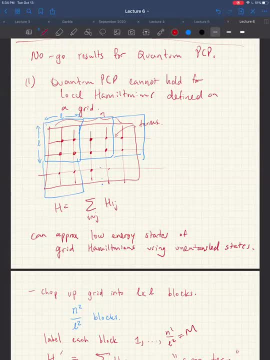 they're. they're too simple, um, to be the types of hamiltonians, that which I'm sure would be like most interested in. So just to get it straight, So we basically solve this problem in polynomial time, deterministically in the case that we have a grid. 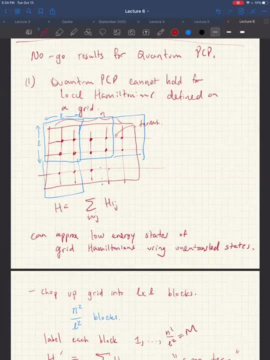 because in the yes case we can find a certificate that says that we are far from the no case in polynomial time. Oh okay, Thank you. Right, So grid Hamiltonians are too simple for yeah. for quantification Henry can, because there are like: 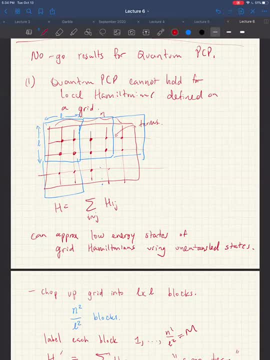 there are like- probably like again- algorithms which use things like that And they consider some of these boundary terms or like the crosstalk, And but then they are able to get like, at least for a few people, like there has been a few papers. 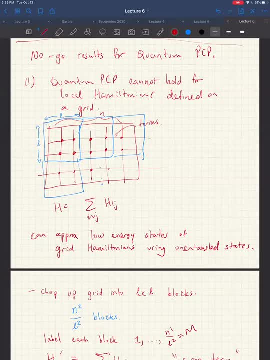 which actually proposed this kind of doing: spreading the whole system into smaller blocks and then trying to correlate them later And they're able to get like pretty good approximations to the ground state energy. So like what does that tell you here that that is a good way of solving like the ground state energy? 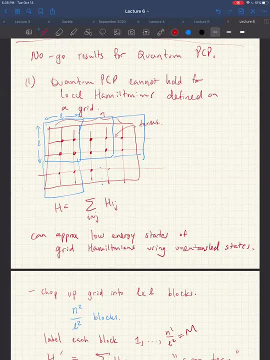 of any K local Hamiltonian, right, If the interactions are neatly arranged in this grid like structure, So like basically you don't need a quantum computer if that, but anyways you can like break down these interactions into just local, but anyways. 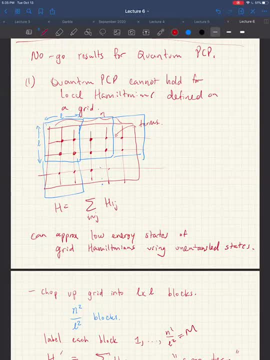 you only have local interactions, right When you're going to run this on a quantum computer or something like that, Because you, when you want to correlate two things that are far apart from that, you break them into like just nearest neighbor interactions. 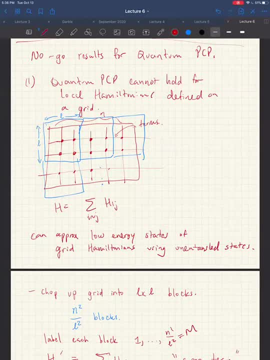 And like you might end up paying extra depth or extra gates, gate depth or something like that, that still works, right? Well, it's whether something or not. I guess it depends on how accurate you want your answers to be. Yes, exactly. So can we say something about the? 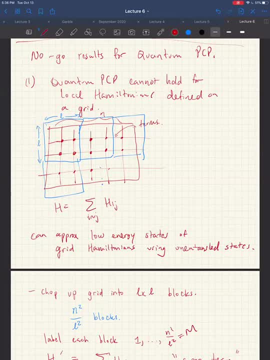 how good your actual ground state energy would be if you use something like this, based on classical, just classical approximation, or classical methods or something like that. Let's see. So I guess I'm not sure on this distinction being class. So here I'm. 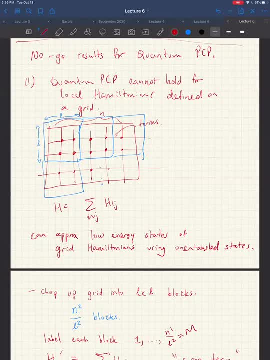 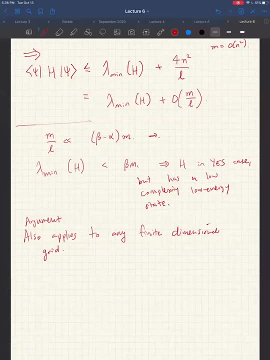 talking just about a classical method to solve this, And the result is okay. so it's a solution. but what is the quality of the solution? It gives you an additive error of M divided by L, And for, in many cases, this is: 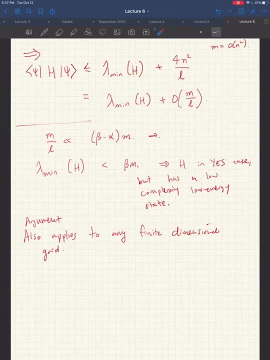 this is like too big, Big of an error. Okay, Right, So oftentimes you want to do much, much better than this, for you know, if you actually want to solve this in practice, And but the but the uh-huh. 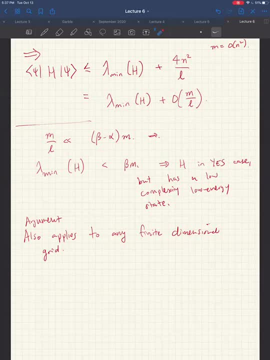 So like, yeah, okay, So like, exactly like, so like, because the like. there is a literally an exact quantum algorithm which does this, which basically breaks the grid into small blocks and then transform, once you have. 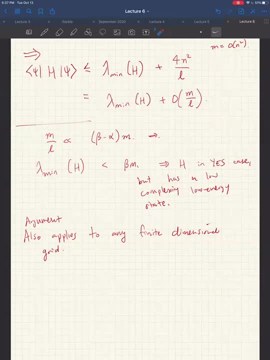 Solved these small blocks. it transforms the Hamiltonian, or like to take into consideration these crosstalk between these two blocks And like. so basically, that algorithm almost gives you the same effect as the classical algorithm, or something like that. or is there even a need for? 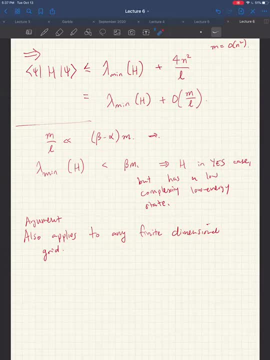 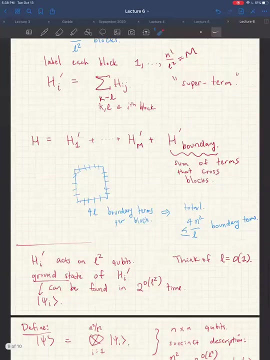 like a quantum algorithm for this case Probably. Oh, I see what you're saying, So I'm not so familiar with the quantum algorithms for this. Um. well, I can't say this though: Um, in general, you won't be, even with a quantum algorithm. you won't be able to solve these 2D. 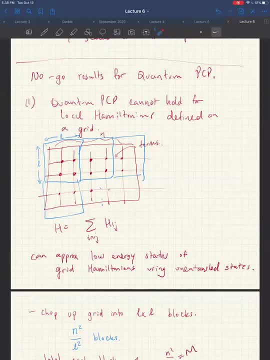 grid systems, exactly Like you won't be able to find uh approximations to the ground energy that are, say, inverse polynomial close to the true answer. And that's because, uh, these grid, uh Hamiltonians are still complicated enough that you can put QMA complete problems on them. 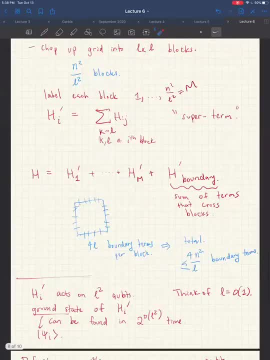 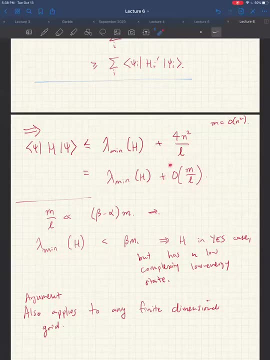 Okay, It it so. so really, here, the the distinguishing thing is, you know, is what quality of approximation you're willing to tolerate. If, if you, so, if you want a very, very good approximation, then then even a quantum algorithm won't help you in polynomial time. 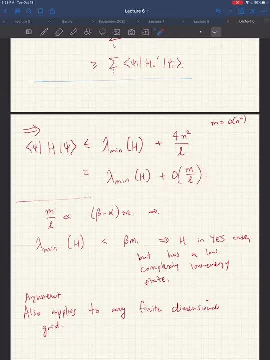 But we're saying: if you're willing to tolerate a very coarse approximation, something as big as M over L, then there's a polynomial time algorithm to do it for you, Okay, So basically, uh, if you're like, it depends on the threshold of error that you're. 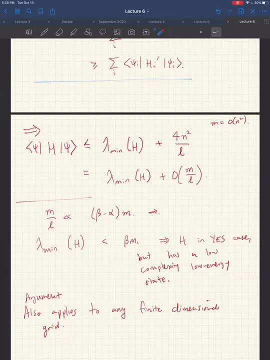 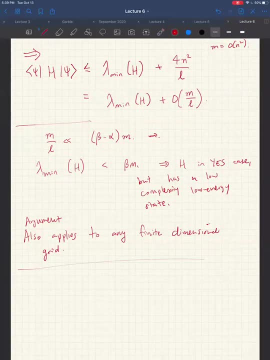 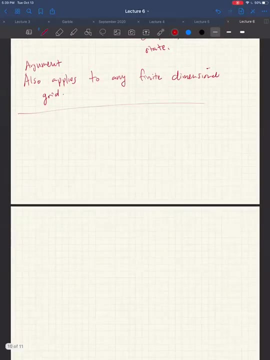 willing to accommodate. Yes, Yeah, Okay, Yeah, Thanks, Yeah, Very good question. Um, okay, So, um, let me move on to the there's. there's one more no-go results to- to kind of illustrate something that's different: Um, so this, uh, you know basically. 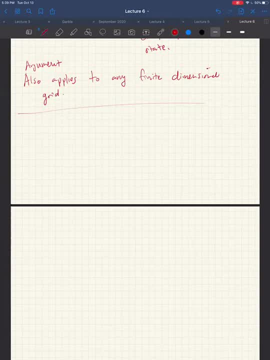 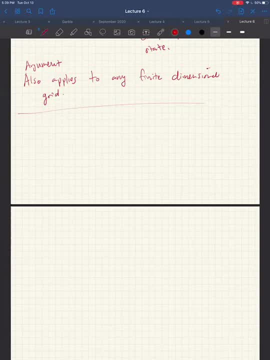 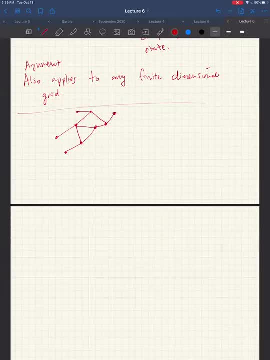 here's some graph, right, So the qubits sit on the vertices and the edges connect the the different vertices. Um, but if your graph is decomposable, where you can, you know, chop it up into small pieces and then there's very few uh terms crossing uh the pieces. 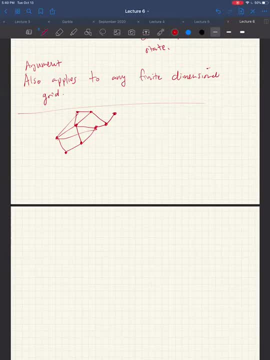 then you could. I mean, the same argument holds right. this isn't so from a complexity theory point of view. this is not so surprising because actually the same argument holds for the, the classical PCP theorem as well. right, I mean it's saying that. okay, so we know the classical PCP theorem is true, it's. 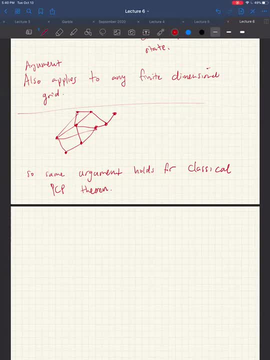 it's proved and the result you know it produces these, the theorem produces these very interesting constraint satisfaction problems like these, three set instances where you know it's hard to tell whether you know half of the clauses are satisfiable or almost all the clauses are satisfied and the these 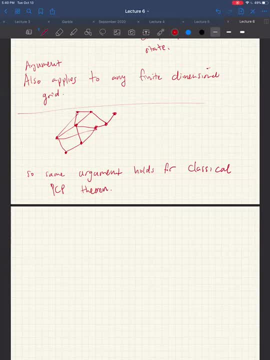 three set instances that are produced by the, the theorem, are not going to be on this grid for exactly the same reasons, and in fact they, the these, these three set instances, will have a much more complicated system of interactions. right, so you know. you look at all the clauses and the constraints in the in. 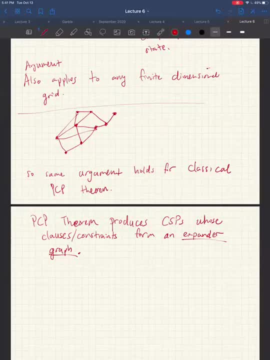 these CSPs and how they connect to the different variables and it forms a graph and these graphs are going to be very highly connected right, and they're going to form what's called an expander graph. expander graphs are those that it's basically impossible to you know decompose it into small pieces. 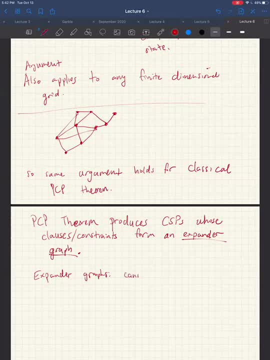 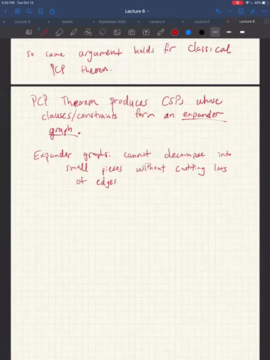 without cutting a lot of edges, okay, so, So you know, knowing this is what the classical PCP theorem produces, you know you might be inspired to say, well, maybe we can engineer local Hamiltonians where all the interactions lie on an expander graph. 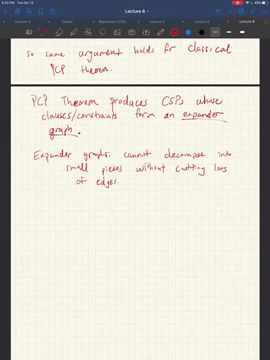 And maybe that's the way to go, And you know, this is a very natural thing, But what's funny is that it only if you go too far it actually starts backfiring Right. So so classically. 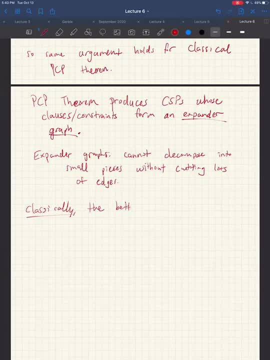 The better expanding your interaction graph gets Meaning, the more highly connected it is, The better PCP theorem you can prove. So what I mean? that like, as you increase the, The expansion Properties of your graph, Then the resulting classical PCP theorem that you get has better and better parameters. It's like a stronger statement. 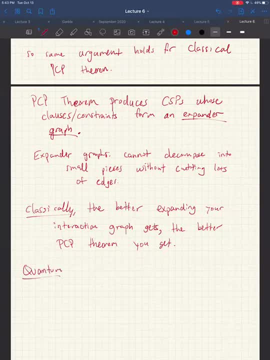 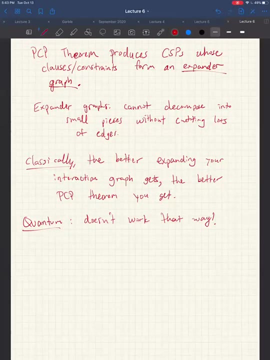 But quantum way. This is not the case. So this is a very, very like you know, initially this was like a very counterintuitive result, saying that actually, if you had like a system of like a local Hamiltonian whose interactions are sitting on an extremely good expander, it's actually also not. 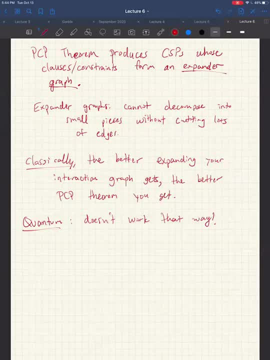 going to be that complicated, like you can also find ground states that have pretty short descriptions. so so here's a, and this was shown in a theorem by Brandau and Harrow, and and they said: you know, suppose you had a two local Hamiltonian, so the okay. so you basically have interactions between two qubits. 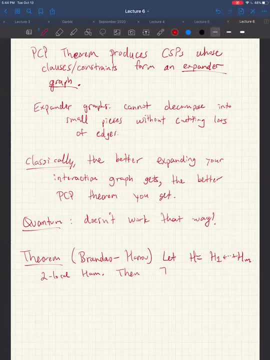 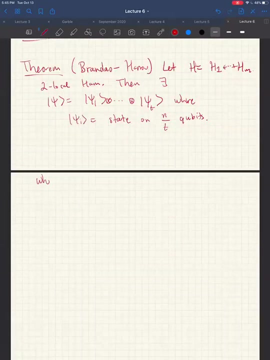 each. then there exists a product state, okay, where each psi i is a state on some small cluster of N over T qubits where the energy of this product state is actually going to be pretty good. it's going to be the minimum energy plus something related to how good of an expander your graph is where. okay, what? 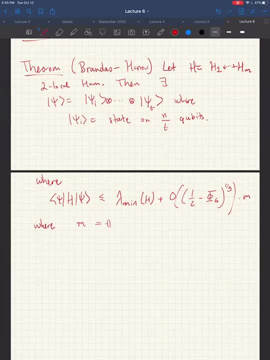 are these? what are these numbers? so M is again the number of terms of your Hamiltonian and this Phi. so G is going to be, it's going to be a measure of the expansion of your graph, the interaction graph. G, okay, and, and this, this is a: 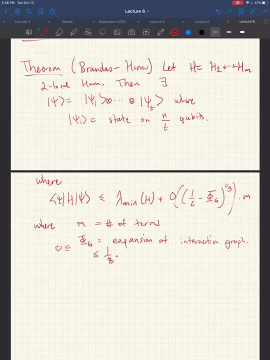 number between one half and zero. okay, so, so this is a theorem that they proved. and as you get a better and better expander, so this is: as you get close to one half, this is going to be better expansion. then this error term is going to get closer and closer to zero, which means you get a better and better. 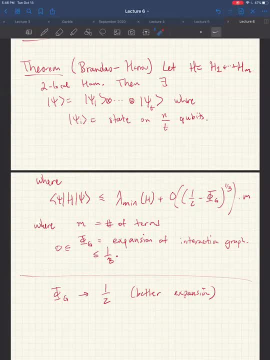 approximation of the ground state okay, but on the other hand, if you have terrible expansion, like if, if you know you, you make this expansion go to zero- then that means you can chop it up into- you know your interaction, graph into small pieces and then you can use the same art. you know the argument. 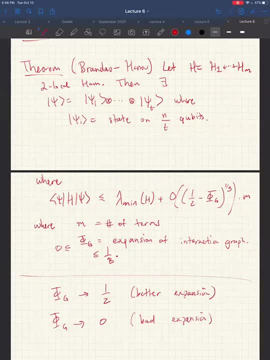 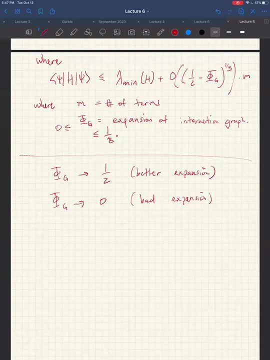 that I presented before to get also a good product state. approximation of the ground state: okay, so you know it's kind of like a weird lose-lose situation. so does the intuition behind this proof come? come from the fact that when you have a good product state and you have a good product state and you have a good? 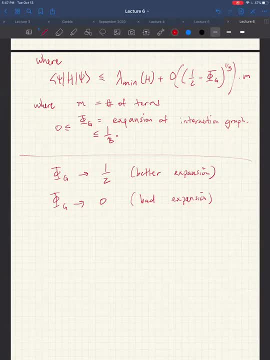 let's say, a lot of these terms are talking to each other, the the influence or the influence that each of them have on each of them is not as great. so, like you have a better expansion or you have better approximation, but when you have like very few terms that talk like between these blocks or between these, 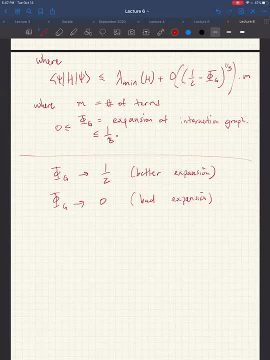 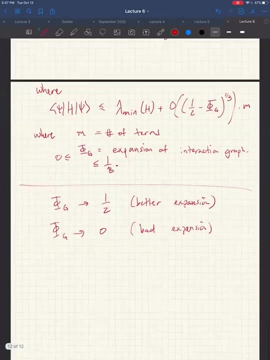 two like graphs or something. you cannot neglect them. so like, if you neglect them, your approximation is bad. that's right, let's see. so this statement is sort of saying that you, at least in in the one half or zero regime, you get good approximations. it doesn't say anything. 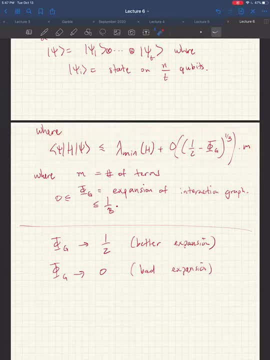 about having bad approximations. so basically what I meant was like, let's like, because when you are saying better expansion, like when 5g approaches half, it basically means you cannot construct a better expansion. if the 5g approaches 30% half, it basically means you cannot construct a. 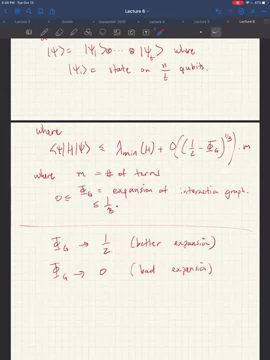 Asim Kadavig- Blocks right, which are without cutting terms, without like neglecting some of these Hamiltonian terms that act between these two sub graphs, Right, right, So does like Asim Kadavig-. My question was: does seem to like, if I have to think about, by this is the case that when, when this is the case, when you can cannot cut and there are a lot of terms, 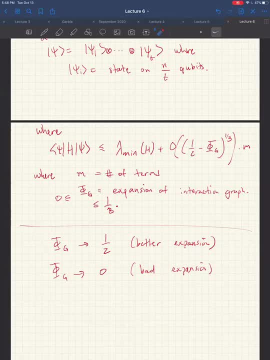 Asim Kadavig- Does the physical motor? or like, if I have to think in the physical dumps, like, because there are a lot of terms that are like doing these crosstalks between these sub graphs, Like that's why the, the 5g, or like that's why it's hard to like, separate them, So to to have an approximation, That is good. 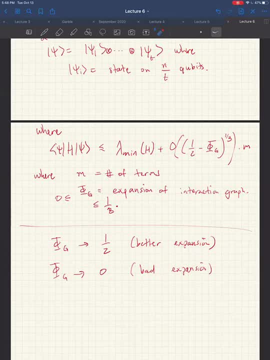 Asim Kadavig- You can basically neglect some of these terms because they might be, they might come into effect because of some other terms that are already in place. Asim Kadavig- Being considered in some other graphs, but when, when, when the case, or when you cannot separate these- the full graph- into smaller graphs. 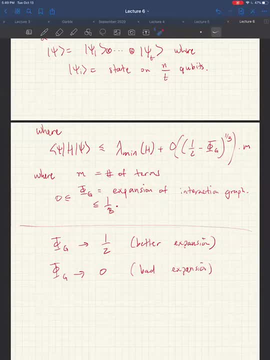 Asim Kadavig- And like there are only a few terms, Asim Kadavig- That that are there. So, like you can you know have to cut, or you know have to neglect very small number of Hamiltonian terms between. are these sub graphs then these? these have higher effects on the, the approximations that you make. 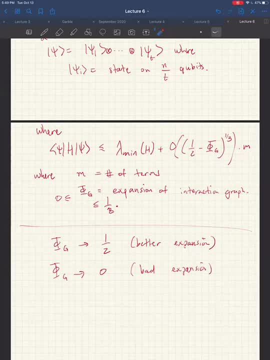 Asim Kadavig- Mm. hmm, So I mean it sounds reasonable. But one thing to notice is that your art, you know, the intuition you're providing somehow isn't taking into account whether your system is classical or quantum. So we know that. 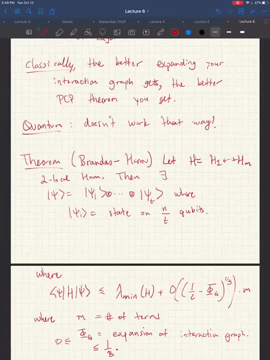 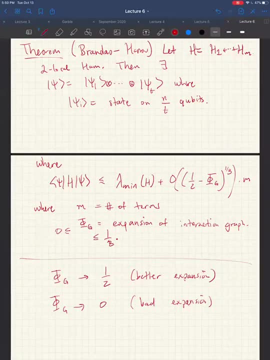 If you have a classical constraint satisfaction problem, or in other words like a classical Hamiltonian, Then As the As the expansion gets closer and closer to half, it's actually harder and harder to find good approximations to the, You know, the lowest energy state. 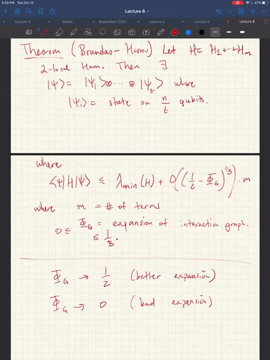 So, So really, what's happened? What, basically, what's happening here is kind of like a genuinely quantum phenomenon. When you have, like, more and more Connectivity between your, your image Interactions, it actually forces. Basically, the upshot is is forcing your ground states to become more and more classical. 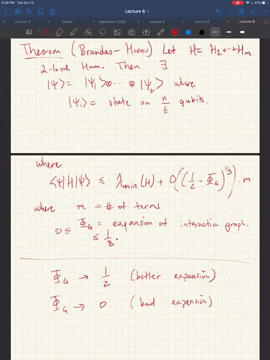 Asim Kadavig- Yeah, Asim Kadavig-. So because, like in chemistry, like when, when we talk about these correlated system, So like when you have these electrons that are like there are a lot of these correlated system where you have, let's say, a lot of. 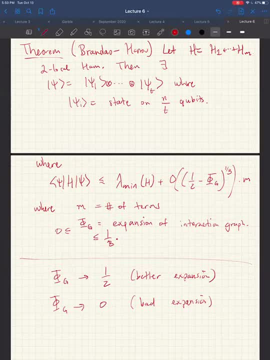 Asim Kadavig- Or there are terms which are very important if you neglect them. Asim Kadavig- Like, imagine Asim Kadavig- All these electrons sitting on a grid and there are these highly correlated systems where, if you neglect one of these terms- So like if you wanted to do an approximation, where you wanted to consider a product state, where you did not consider a crosstalk- 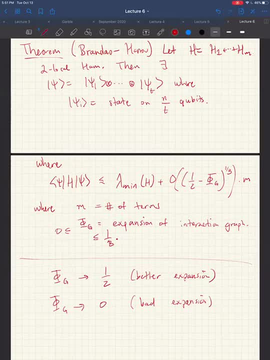 Asim Kadavig-. That would lead to very bad approximations because it's like, literally the opposite case of like. if you don't consider the full Hamiltonian terms, your approximations would be very bad, Asim Kadavig-. And on the opposite side, when, like when they are not highly correlated. 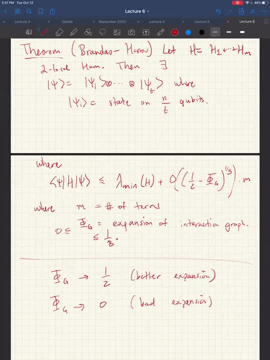 Asim Kadavig- Systems. then yeah, like yes, sure, If you consider a product state It's, it works pretty good. Asim Kadavig-. So, like Asim Kadavig- This was, this is exact or this is kind of the opposite. 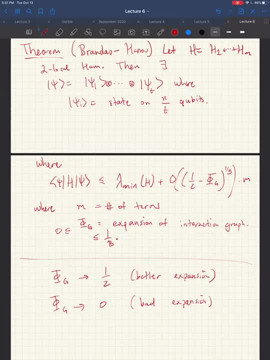 Asim Kadavig- For correlated systems and chemistry. just, Nicholas Matsakis- Is right. Yeah, I mean, this is yeah. In some sense, this is maybe a little more surprising, Nicholas Matsakis- But this is really saying like, if you, if you pack in a lot of cross terms. 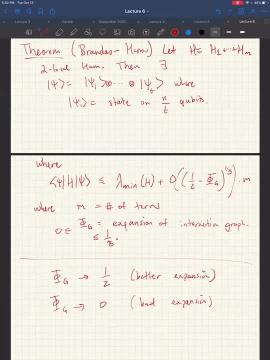 Nicholas Matsakis- And I think like sort of, maybe way more than what you might encounter in in quantum chemistry or something, Nicholas Matsakis- Then it says that you can, Nicholas Matsakis- You know, to use some physics terminology, that these mean field approximations are actually quite good. 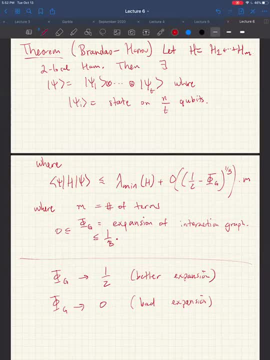 Nicholas Matsakis- Mean field means like product state approximations, Right, Nicholas Matsakis-? And that's what's really behind this theorem is that once you're you're in Nicholas Matsakis- Your interactions just getting really, really dense and highly connected. 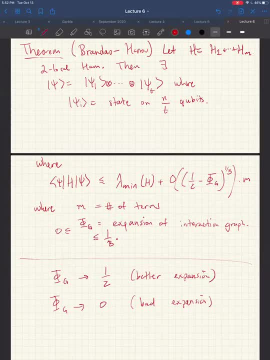 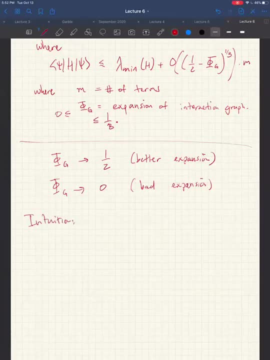 Nicholas Matsakis- You don't, Nicholas Matsakis- Your ground states don't need any entanglement. so, Nicholas Matsakis- So so the intuition comes from this thing that we've discussed earlier, which is this monogamy of entanglement. 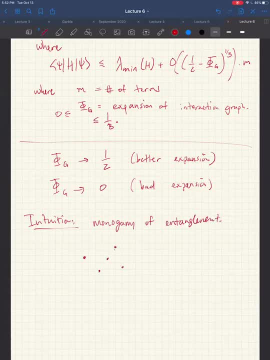 Nicholas Matsakis- Which says that you know, if you have a bunch of particles, but they're all like, they all have constraints on all of them, Nicholas Matsakis- And you know, you can think of each of these constraints as saying, oh, we all want you to be maximally entangled with each other, but but that's not possible. The only way to sort of 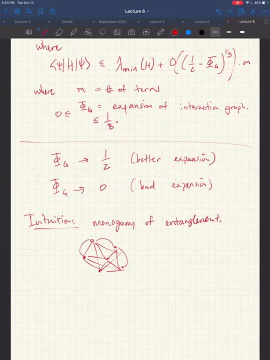 Nicholas Matsakis- I mean, there's no entangled state, that's, you know, satisfies all of these constraints and really they just forced to be product states tenants. Nicholas Matsakis- So how about graphs that have very bad expansion but you cannot decompose into small pieces? For example, take a quick fake and not a, not another quick connect, connect, connect them by an edge. 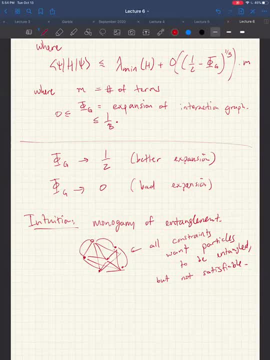 Right, Right. so then you can sort of like interleave both arguments. you just divide. you know, you chop the two clicks in half and then you know that this click and this click are super good expanders, and then you just sort of find the product state approximations for both. 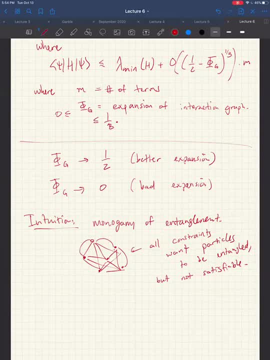 and then, Yeah, sure, but like now, let's say, you have square root of n clicks and you connect each one by an edge. Yeah, I think you know here. okay, so the point here is that we're actually willing. 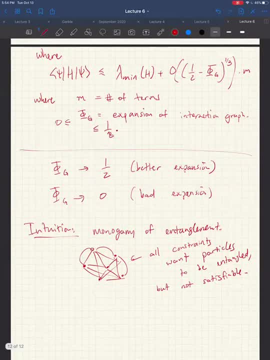 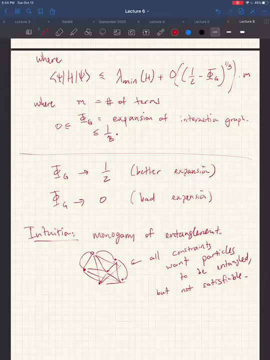 to tolerate a lot of errors, like a constant fraction of the number of edges. So you know you should keep that in mind. So if you have a lot of clicks but then you connect them with single edges, that you know, the number of interclick connections is relatively small compared to the total number of edges. 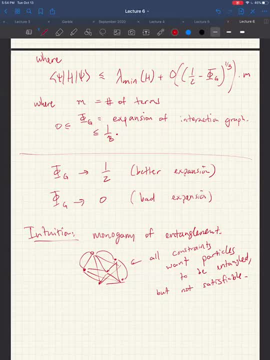 in this entire graph. It's about the same. It's about the same asymptotically, because you have square root of n clicks. you connect one edge between each pair of clicks and each click contains also a layer in n amount edges to it, n inside and n outside. but maybe that's still. 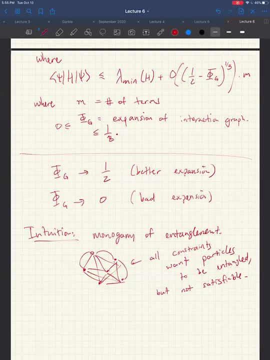 Okay, so yeah, but you're basically homing in like: can we find examples of graphs for which maybe we can noodle our way around this? That's possible. so you know, I guess the punchline is that we've at least identified. 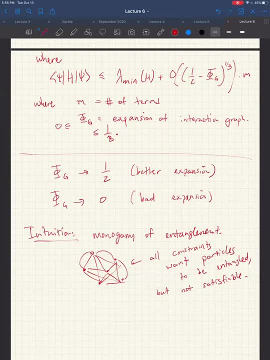 the extreme ends of which we know it's not possible and we're really looking for some Goldilocks solution where you know it's expanding but not too expanding. The main lesson that this theorem of Brandeau and Harrow is telling us, and there's like: 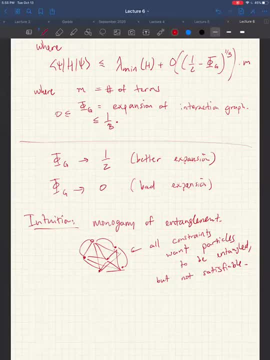 a related theorem that says actually also, your graph cannot have too high a degree, like a particle cannot talk to too high a degree. Yeah, The particle cannot talk to too many other particles, exactly for this monogamy of entanglement reason. but of course, like you said, it's easy to come up with graphs. 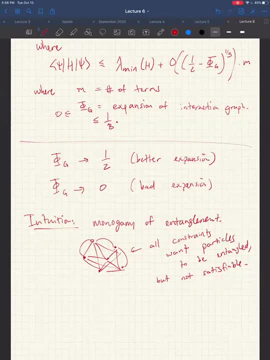 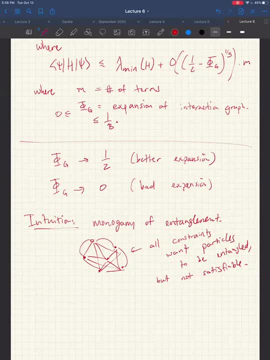 graphs with degree four or five, but there are not that well connected Right. So it's possible, and this is not covered by the theorem of Brandeau-Harrer. But you know there's still some sense that this would be too easy of a solution. 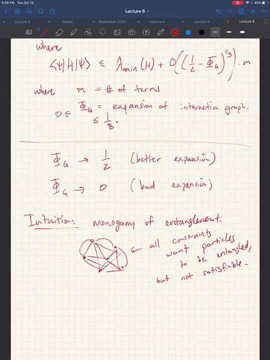 and you say, oh, let's just make the clicks a little smaller, and so on. Okay, But you know, we don't know. So this is basically what we know about quantum PCP, which is to say not much, but I think. 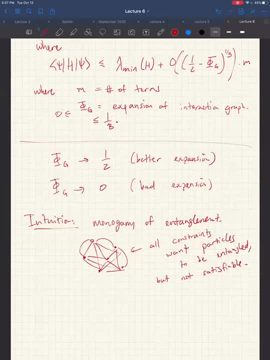 it's really intriguing, like: basically can we imagine and come up with really exotic types of local Hamiltonians that have really exotic low energy states, that exhibit all sorts of weird entanglement, and basically the best candidates for such weird Hamiltonians are ones that come from quantum error? correcting codes. 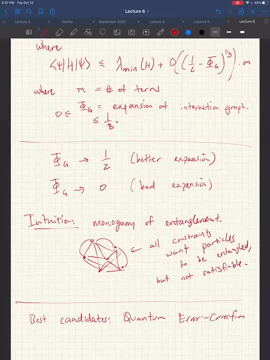 Quantum error correcting codes give rise to Hamiltonians and so and we sort of by definition, the quantum error correcting codes have to create states with really really robust forms of entanglement, right? so by definition. So it seems like a good place to start and really that's what people are looking into. 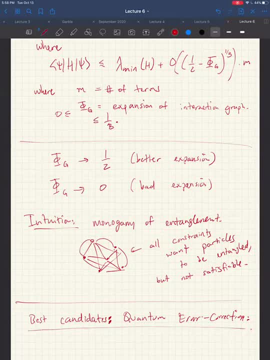 But yeah, you know the story is still open, Okay, so basically we've reached the end of the part of a class on Hamiltonian complexity And yeah, so hopefully you know you got it, Okay, Thanks. Thanks for taking time out of your day to kind of get a sense of the lay of the land. 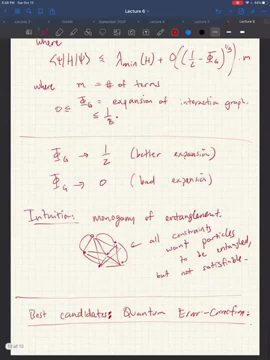 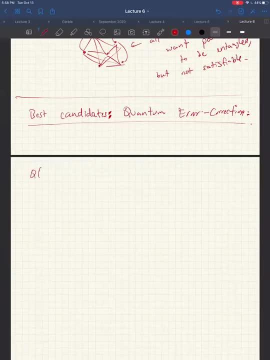 I was gonna, you know, if I had half an hour left. I was going to start a section on QMA II, but I might, you know, move this to next time, But maybe not. So the next, you know unit of this class will focus, sort of will switch gears. 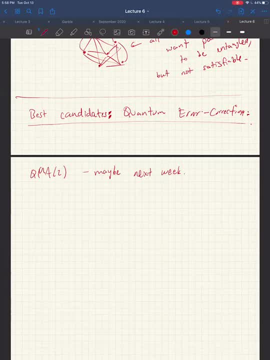 We're not going to talk much about Hamiltonians anymore, although they'll actually make an appearance in the next class in certain places, but we're going to talk about something called the verification of quantum systems and the things related to that. So, yeah, that's it for today. 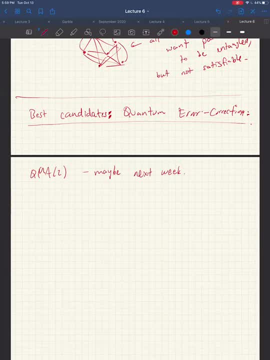 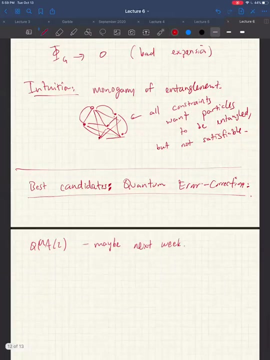 Is it possible that the set of all local Hamiltonians that can be represented by graphs- so I guess two local Hamiltonians, aren't complex enough for this quantum PCP conjecture? Yeah, I didn't mention this, but you say: well, why do the interactions? 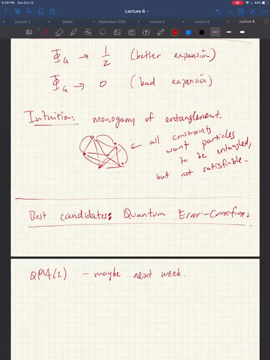 have to only involve two qubits. Why can't they involve three? And we also don't know very much. we don't have any barrier results there. Yeah, I mean especially all these error correcting codes. the interactions involve a small cluster of qubits, Definitely not two. So you can also say that this theorem 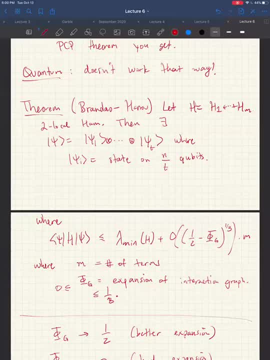 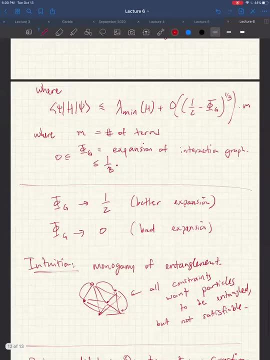 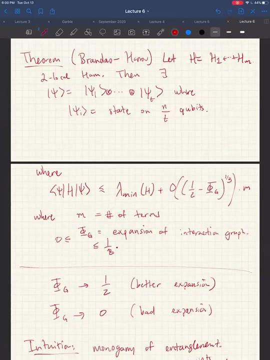 this Brandau-Haro is really ruling out a very, very narrow class of graphs or local Hamiltonians. I think that's probably definitely clear. I guess something that a lot of people are excited about nowadays is this theory of high-dimensional expansion- Expansion not just on a graph, but I guess some 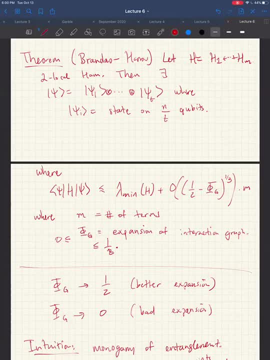 high-dimensional, some functional, complex. Have people looked into that in relation to quantum PCPs or is it wide open? It's wide open. I have a very, very strong feeling that that's pretty intimately connected to what's needed to move forward on this quantum PCP. 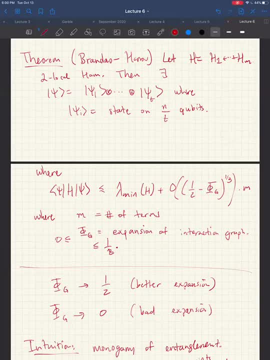 These highly structured, these high-dimensional expanders are kind of like on the border between like being very structured but not too structured objects, And that's sort of the feeling is that you need something like that straddles the borderline to really construct these local Hamiltonians. 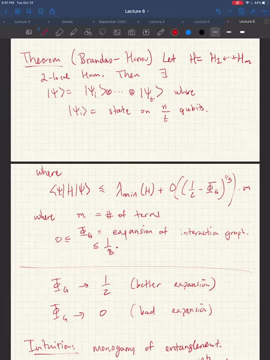 But I guess we're also seeing that high-dimensional expanders are useful for other things not related to quantum, So I think it's, yeah, really interesting. Is there an analog, of sort of a gold-vessel-shape-cell theorem for QMA2, like round reduction? 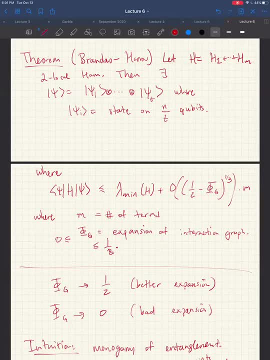 like in terms of public coins versus private coins? Oh, QMA2.. Yeah, so I didn't get into this. but QMA2 here refers to the model of QMA, where Merlin sends you two proofs that are promised to be unentangled. 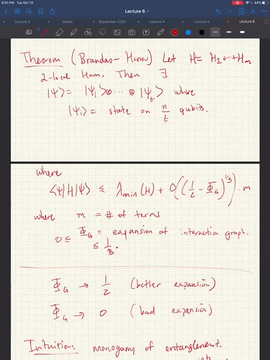 Oh, So it's not a one, it's not an interaction. It's not about interaction. Oh, okay, Yeah, But the question you asked is also very interesting. I think what you're talking about is there's these classes called QAM or QIP, with two rounds. 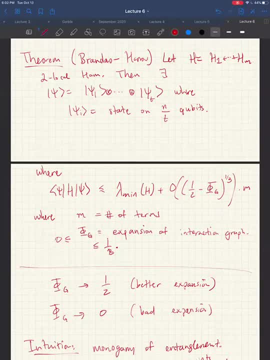 and these classes are very poorly understood, like they sort of no one's pinned down exactly what their complexity is. Wow. So, yeah, I think you're right. I think you're right. So, yeah, I think you're right. 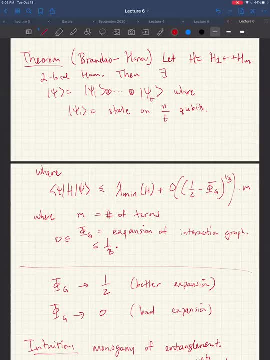 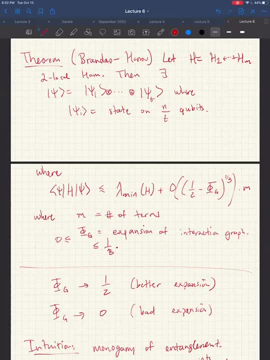 Just to give a preview. so I said: you know, Merlin can send you these two unentangled proofs. And this is actually a very powerful promise as far as we can tell, because in general, if someone hands you a quantum state on two registers, 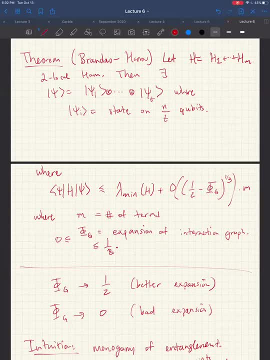 there's no measurement that you can do to detect whether these two registers are entangled with each other or not. So, having the guarantee that the two registers are unentangled, you can actually use that to your advantage, And so one of the things you can do with this is you can. there's a QMA2 protocol for 3SAT. 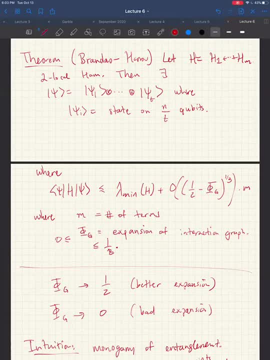 Someone can convince you that a 3SAT formula on n variables is satisfiable, but they only need to send you a square root n sized proof. But if you don't have this unentanglement guarantee, then even if Merlin can hand you a quantum state, 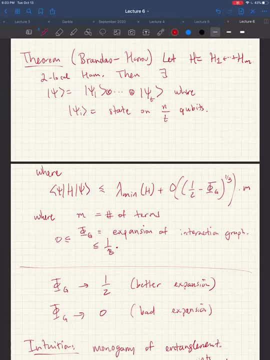 we still think that to convince you of 3SAT they still need to send you n qubits. So with unentanglement you can somehow compress your proof size in certain cases. So, okay, I think I'll talk about this next time.